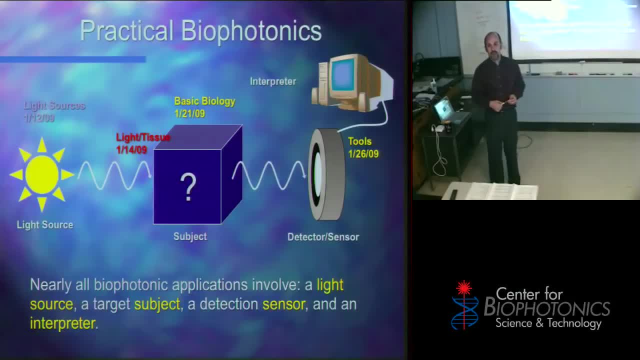 Okay, So we also started talking about how light can interact with matter, And today we're going to continue that by interacting with something called logical repair, And we're going to talk about all kinds of other ways that light can interact with living tissues. 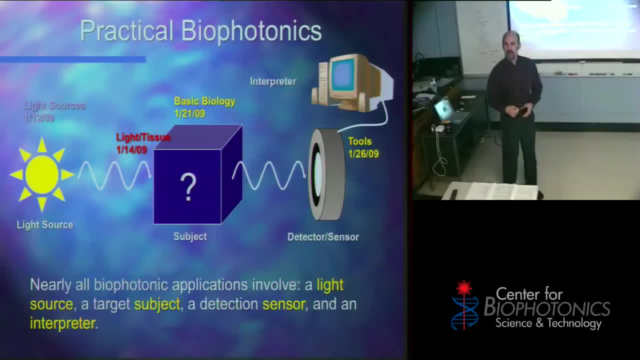 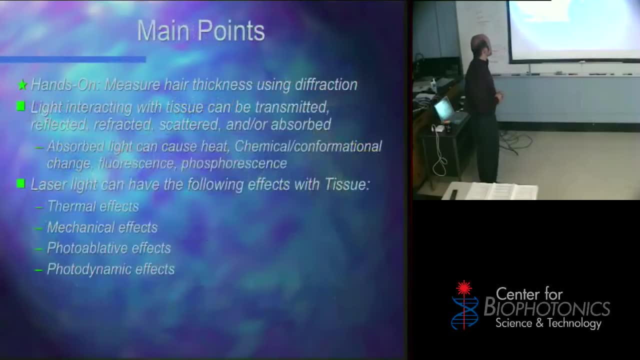 To do things like tattoos and blast kidney stones, things of that nature. Okay, So the main point of the day will be: we're going to measure your hair thickness. Okay, Using diffraction, We're going to look at how light interacting with tissue can be transmitted, reflected. 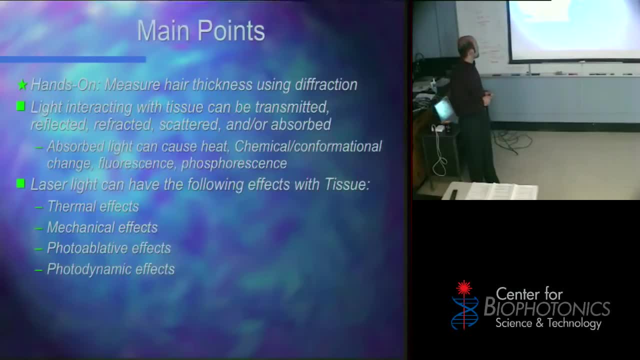 refracted, scattered and or absorbed, And it can all happen simultaneously And we're going to focus in on absorbed light Because that can cause heat, chemical conformational changes, fluorescence, phosphorescence, And that tends to be when photons are absorbed. 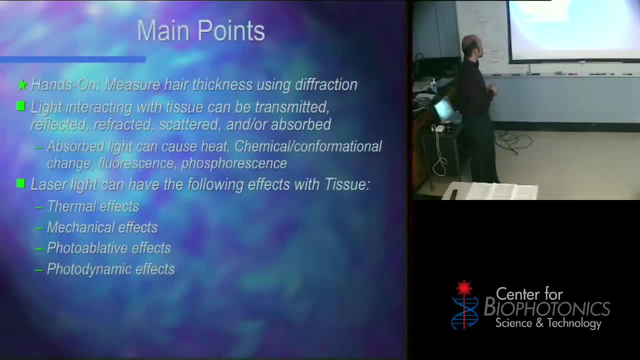 It tends to be when a lot of interesting things happen. Okay, And we're also going to look at how laser light can interact with tissue and have thermal effects, mechanical effects, photoablative and photodynamic effects. Okay, We're going to look at all those four different ways in which laser light interacts with tissue. 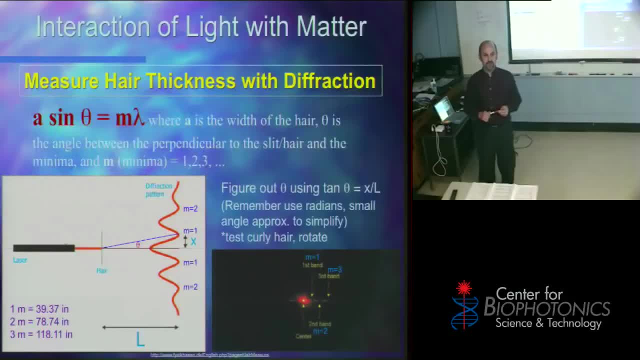 But the first thing we're going to do, probably for about 45, 50 minutes, is you're going to do collect the data for your first lab report, which has to do with measuring hair thickness. Now you're going to see some very high-tech devices out here. 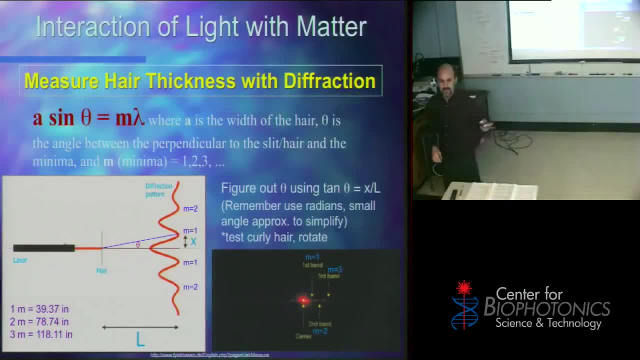 We have Lego laser holders And we have one laser holder. Okay, Just a couple of different iterations. generations of materials: Okay, We have hair card holders And we have hair cards, which most of you already put a hair across one of these things. 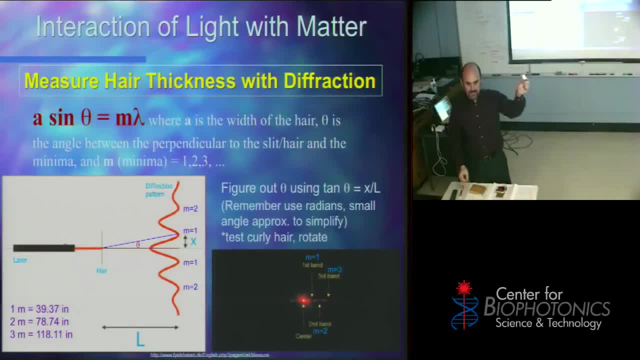 Okay, Now, because I only have six of these, I created another kind like this that you're going to actually have to tape your hair across this, Okay, But I'm sure you guys can figure that out, And I gave you some extra thin Legos as spacers in case you need to move your hair up or down. 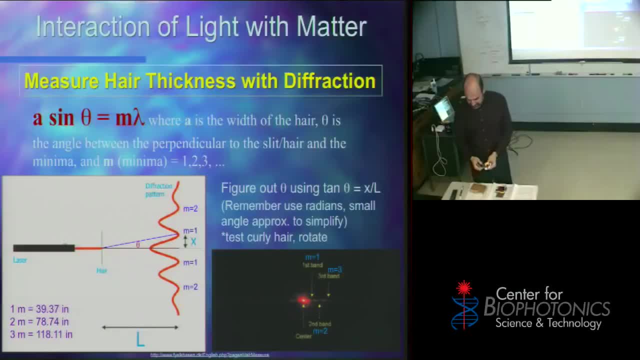 in relationship to how the laser fits on these things. Okay, When you have your card, it's easy because you can move it up and down inside this holder. You guys are going to divide up into eight teams, So there'll be three people on most teams, except one team will have two. 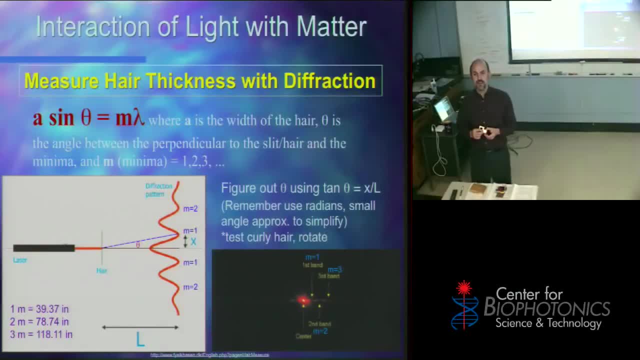 I think, because I saw yesterday there were 23 people. Okay, Okay, Okay, It was an extra person. Let me see, It doesn't look like. Ah, that's what was going on. Okay, I was wondering about that. 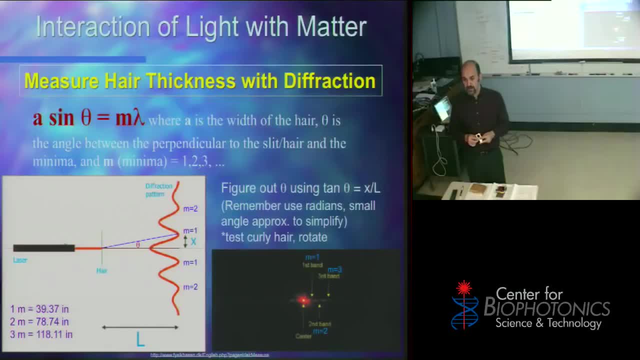 Okay, So actually we have 22 people, So there'll be one group of four, So there'll be seven. So only one of the groups will have to use this approach, And you can use two or three of them if you like. 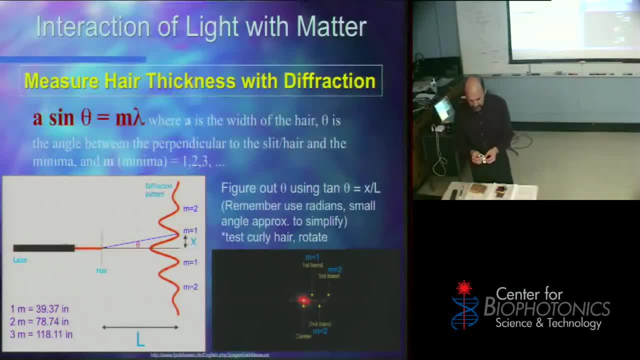 Because you'll have different people in your group. Now, what you're basically going to do is you're going to stick your card inside the holder And you're going to have your laser. There's a spot here for the green or blue laser. 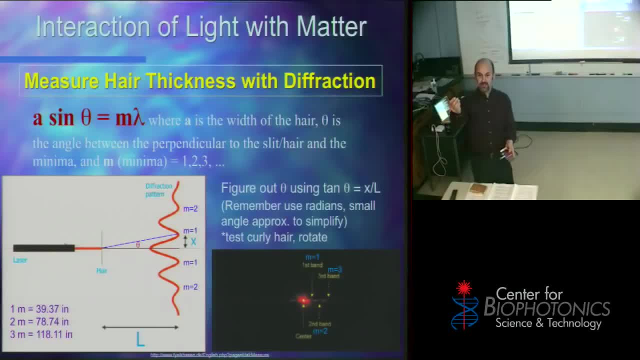 And there's a spot that can be used, also used with red lasers. unless you have this flat red laser, Then you can use it here. You're basically going to measure out a distance, And I'll give you more specifics on this in a moment. 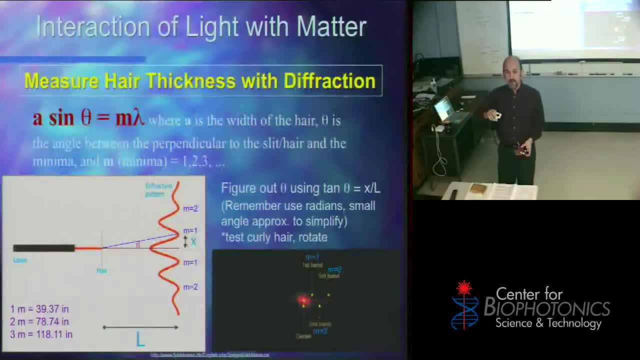 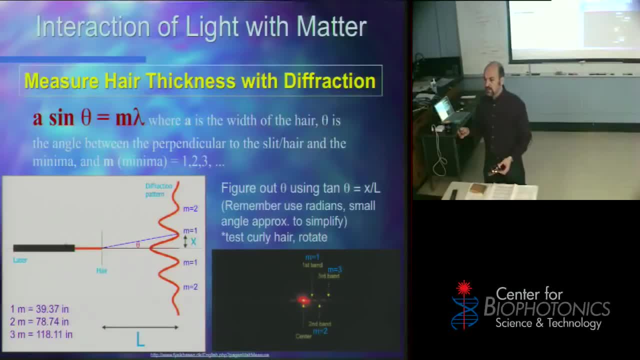 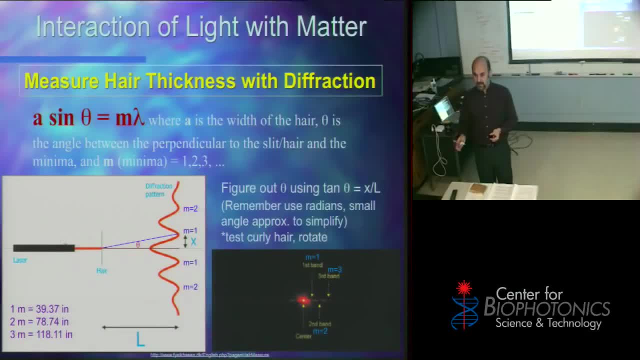 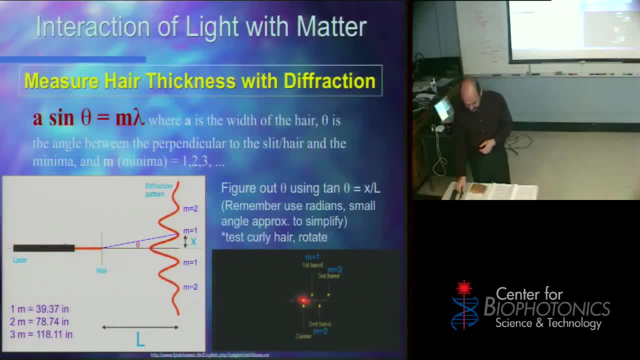 Okay, Okay, These blue lasers. They're much more expensive And I'm going to, while you guys are doing your data, I'm going to pass out three sheets which help you understand how you're going to write up your lab report. 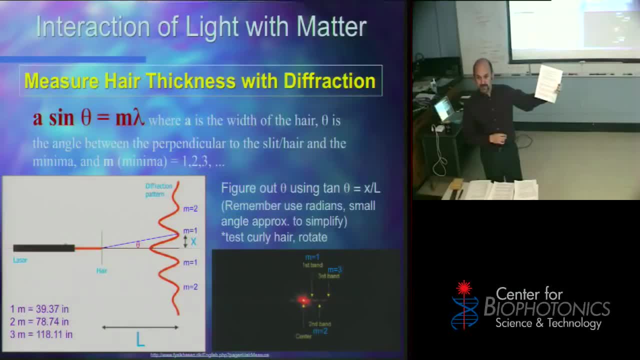 One of them is called the format of laboratory reports. Okay, It explains the dimensions of the labs, different sections that are expected in your laboratory report. It's four pages, big printing. Then there's the checklist for laboratory reports, which is basically like a little cheat sheet. 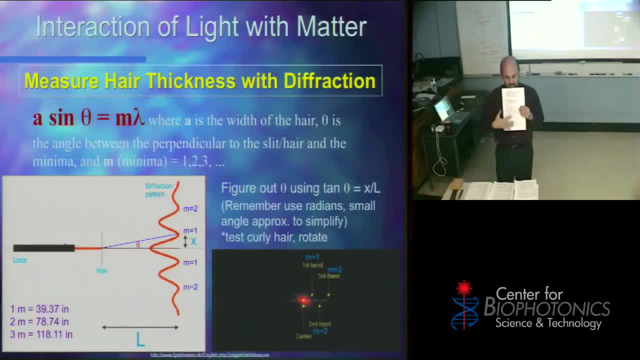 for this. It gives you a sense of one of the main ways in which we're going to be reviewing your reports and how your peers are going to be reviewing your reports. And lastly, we have communicating with graphs, And this one is all about. 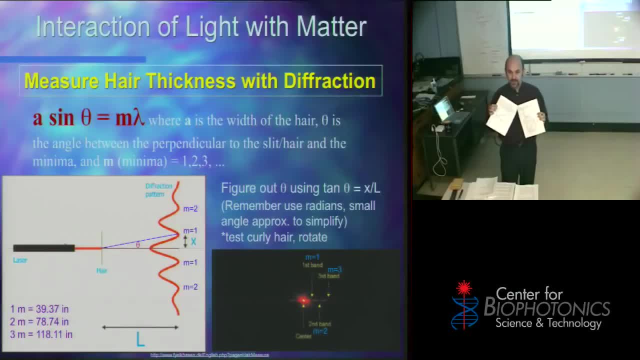 mistakes you can make when you're doing your graphs and things to avoid and things to try to do to make the most effective graphs you can of your data. I don't expect you to follow every single thing in here to a T, but these are. 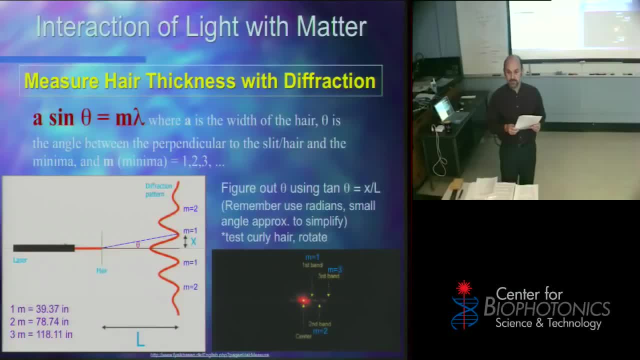 suggestions that will help you get the best lab report possible. I'll pass these out while you guys are doing the experiment. Are these also available on SmartSight? What do your reports mean? These checklists are not right now. I'm going to hand them out to you. 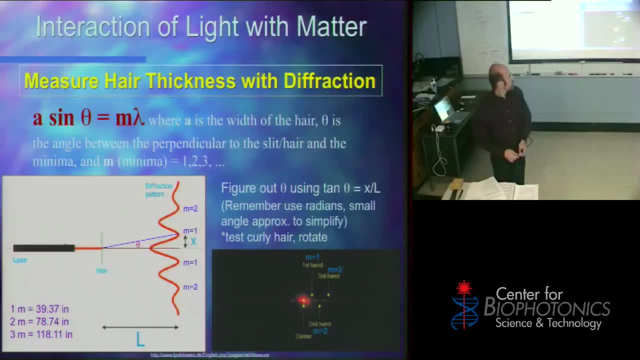 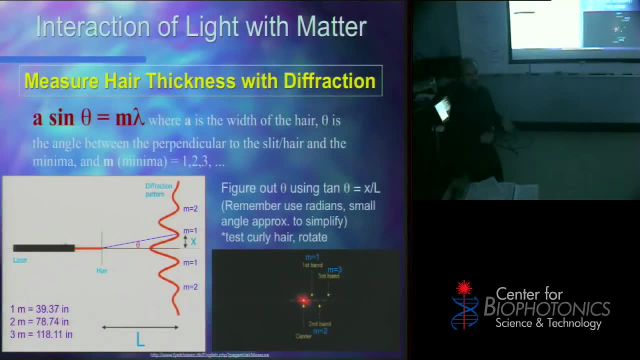 I have to think about that. I'm not sure I want to put them out. I don't know if they're quite yet Okay. so why can we measure hair thickness using diffraction? Lasers give out electromagnetic radiation- visible light in this case. 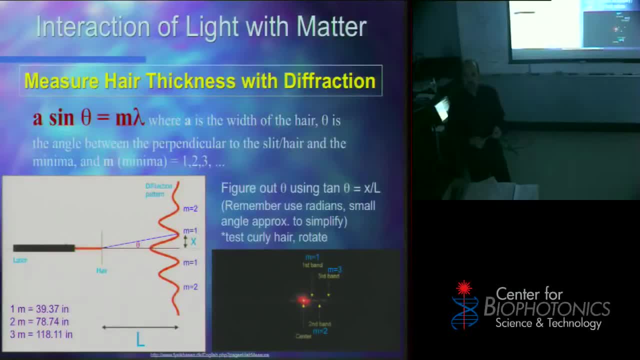 Photons behave as both particles and waves. We're taking advantage of the wave properties of photons to figure out using diffraction and thickness of your hair. You guys remember that if I shine a laser on a hair I'll get a pattern of light and dark. 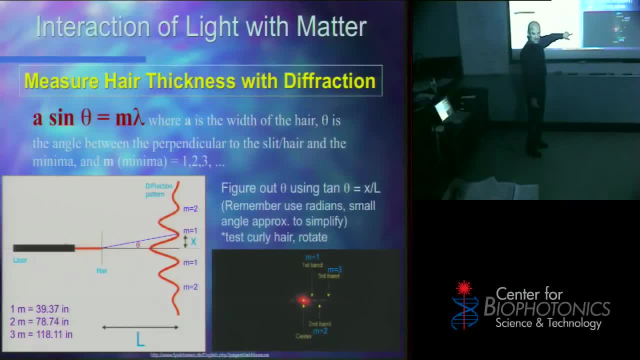 This is supposed to signify light, dark light, dark light, dark. This is just a way of showing that kind of a pattern. This is a actual representation of that pattern. See the bright spot in the middle. Dark light, dark light. 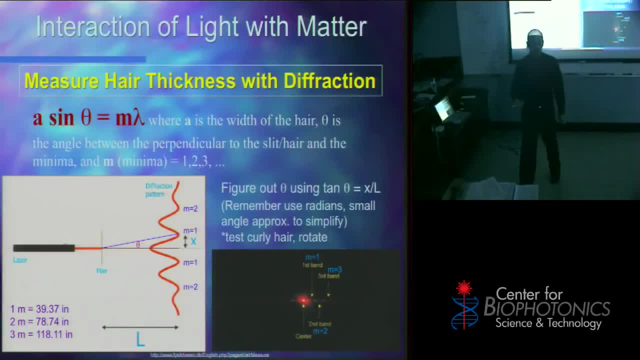 You guys see that Pattern, You guys remember seeing that pattern the other day. Okay, so the equation that tells you the width of the hair is this equation: right here, The width of the hair A times the sine of the angle is equal to M. 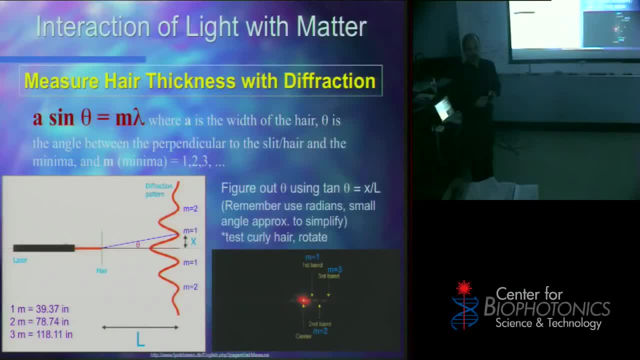 times the wavelength of the light you used. Okay, Let's go through each one of those for a moment. So you're going to try to solve for A. That's what you're trying to find. Okay, Sine of the angle. This is the angle. 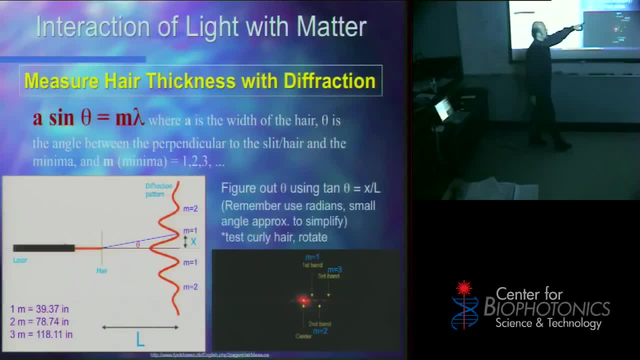 The angle is the angle between the straight line where the bright spot is, straight line that comes this way, and the line that goes from the hair to the first dark spot. Okay, So effectively you've got. I were to magnify it quite a bit. 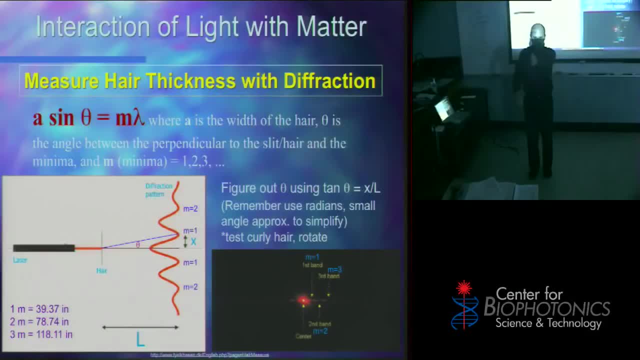 and I'm the hair, the laser shooting from behind me. I've got the straight line that goes where the bright spot is on the screen in front of me, and then I've got the first dark spot and this is the angle. Okay, Sine of theta, That's the angle. 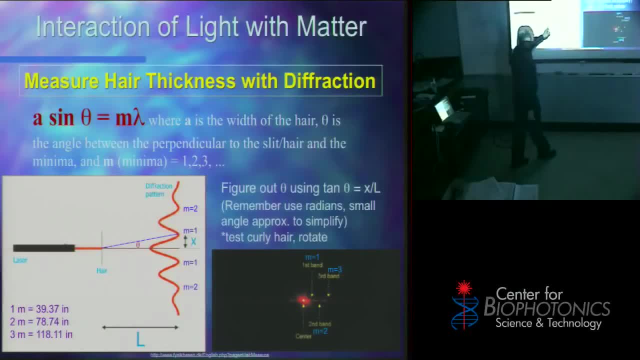 And then that equals to M, and in this case, if I choose to measure the first dark spot, M equals 1.. If I choose to measure the second dark spot, M equals 2.. If I choose to measure the third dark spot, 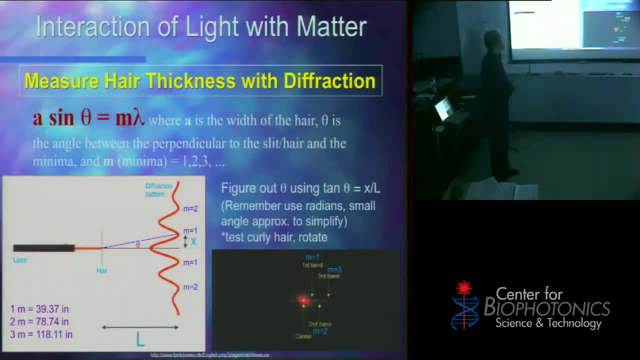 M equals 3.. Okay, Just depends on which one I'm using. Times, the wavelength: The wavelength you can read on the laser. The laser has a little tag and it'll tell you the wavelength. It'll tell you the wavelength here in nanometers. 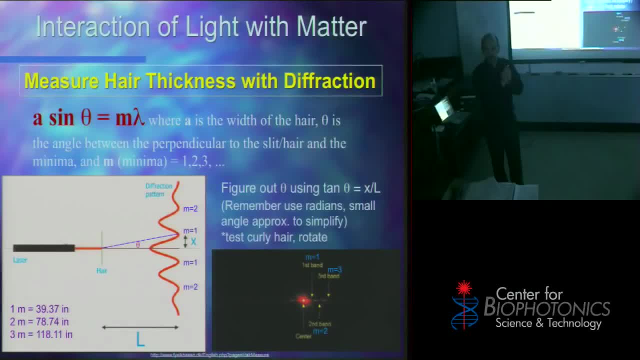 Okay, The really important thing today is to make sure you're consistent with your units. Okay, Now, how the heck are you going to figure out this angle? It's easy to figure out this because it's written on the laser. It's easy to figure out this because it'll depend on: 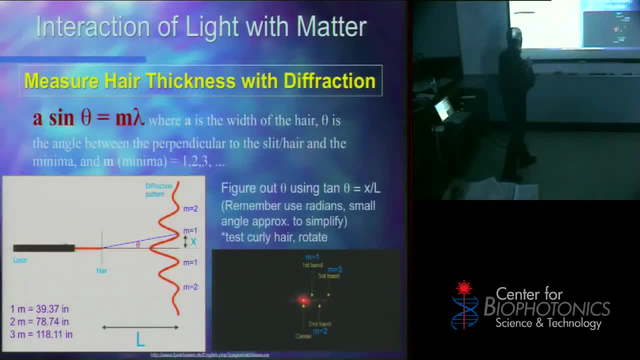 which one you decide to measure. But how do you figure out that angle? Well, that angle can be figured out this way: The tangent of the angle is equal to X, the distance between the bright spot and whichever minimum you're using, divided by. 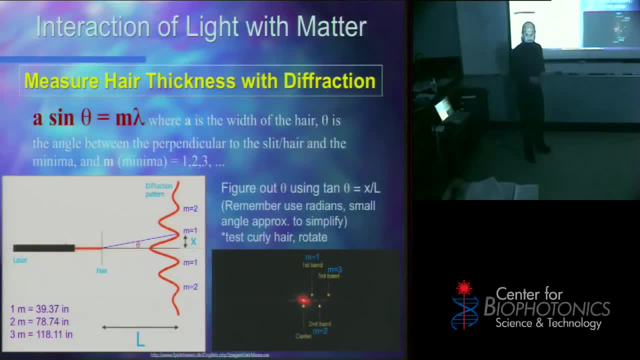 the distance from the hair to the wall. So you're going to have to know the measurement from the wall to your hair and try to be very accurate with that measurement. And you're going to have to have a very accurate measurement of from the center of the bright spot to the wall. 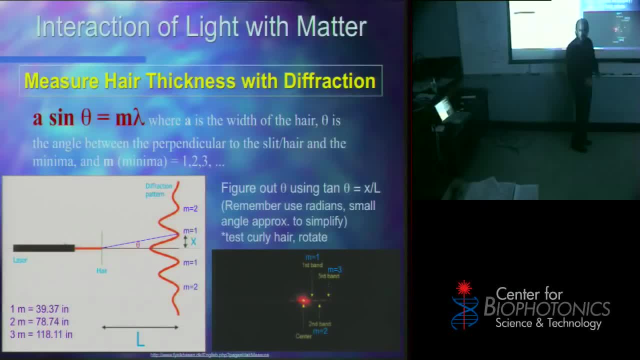 From the dark spot to whether you're using the first dark spot, the second dark spot. Some people will choose to measure from dark spot to dark spot and divide in half. That's perfectly reasonable. There's a lot of different techniques you can use. 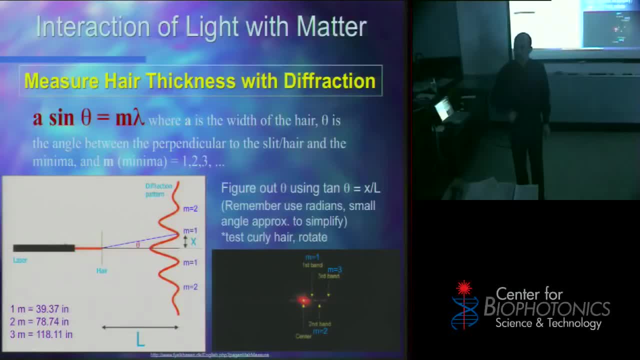 But you have to make sure you write down what you use, because that'll help you in the report. Yes, Are you measuring to where the dark spot begins, The middle of the dark spot? You always measure to the middle, The middle of the center here. 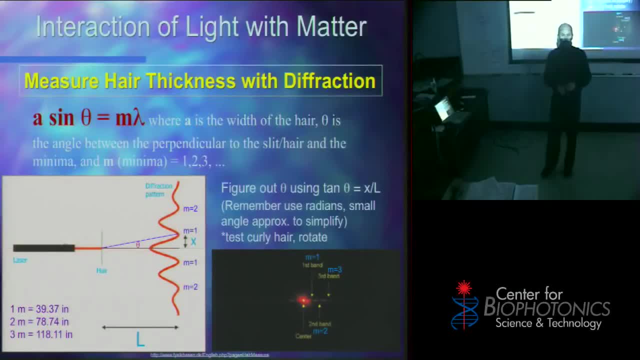 right in the center and then to the middle of the dark spots. Okay, So do you guys think? do you think that measuring the first dark spot will lead to more accurate results, or measuring the second dark spot will lead to more accurate results? 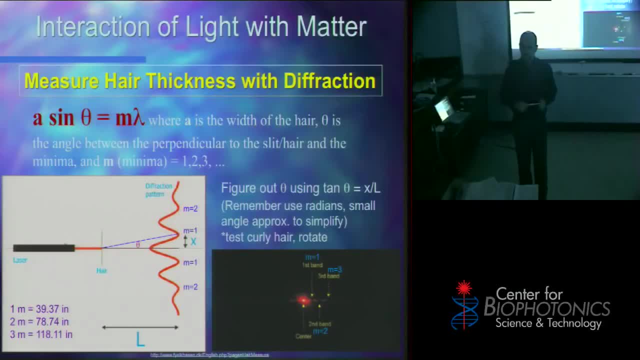 And why. First one is probably going to be easier to find the more arrow or something, so that'll probably get more accurate results. So this is going to depend. okay, We're going to try to make the room as dark as possible. With the green laser you're going to get brighter space. 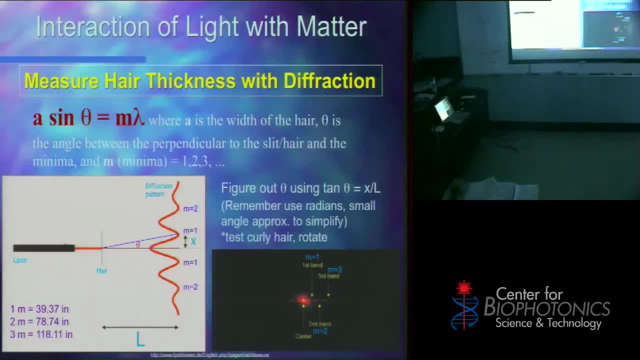 When you're making a measurement and you're using a ruler. when you make a measurement and you make a measurement that's this big versus a measurement that's that big when you make a larger measurement, you're likely to have less error if you can see where the measurement should be. 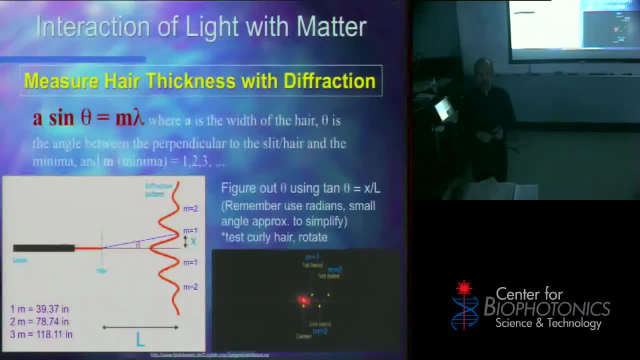 So if the image is bright enough and you can see where that second dark spot is or that third dark spot is, you're going to get a more accurate measurement, because the error decreases as you go out to a larger measurement because of the way the division works. okay, 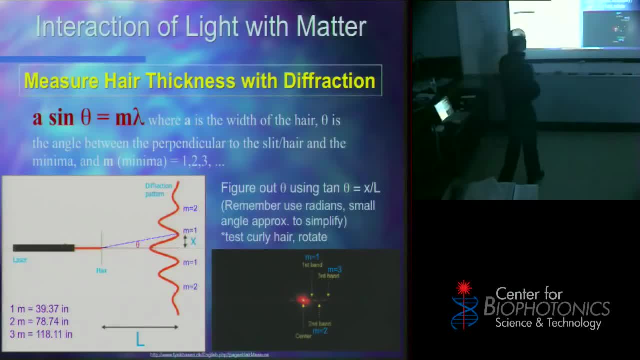 You guys get that. So would you rather be one meter away, two meters away, three meters away? and how might that affect your readings? Well, you can go as far away where it's still very difficult to see. And why would you want to do that? 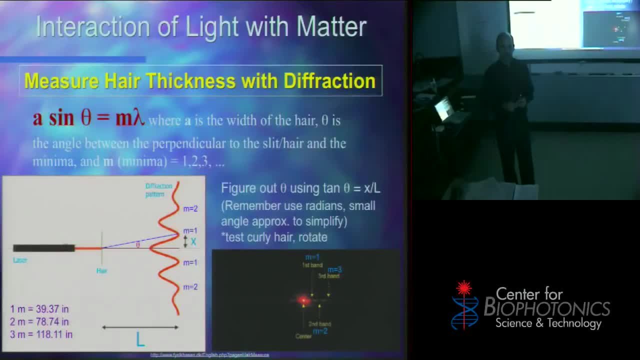 Well, the further away it's the same thing. The bigger it is, the less like the length, the less. this number will be bigger, there'll be less error. and this number will be bigger, there'll be less error, okay. 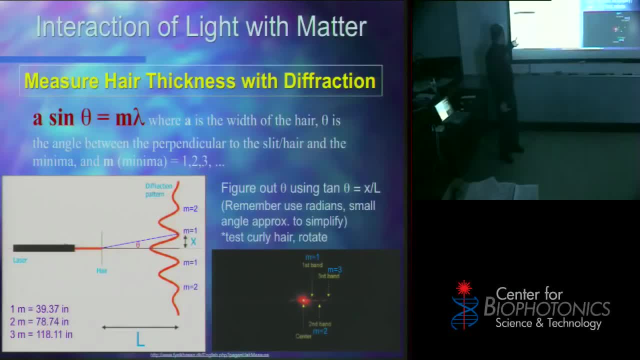 So I've given you- I have two tape measures out there and I've given you. well, one meter is equal to an inches, two meters and three meters. okay, My suggestion to you is to see, while I'm writing this book, 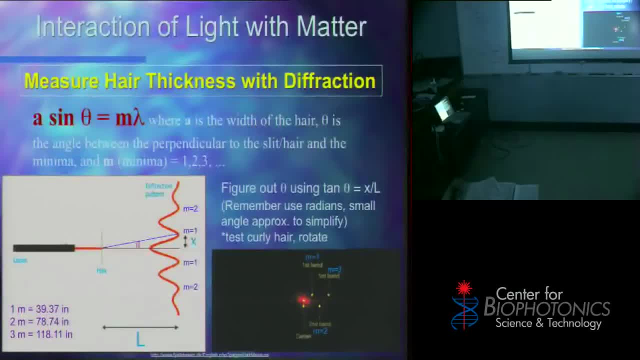 and see how far you can go. These are the two tape measures. They're going to be projected against one of these walls or one of those or one of the back walls. okay, You pick the wall that you want to get down. 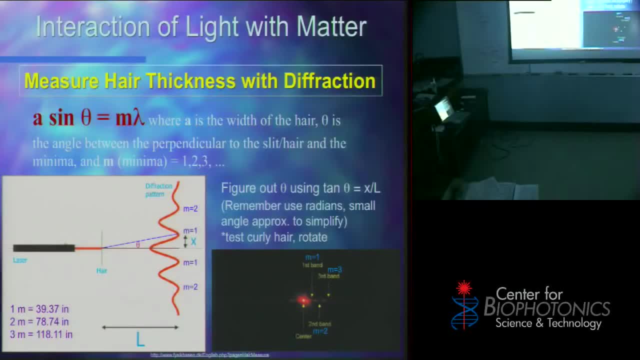 There's some scrap paper over here and there's some- excuse me- some- nice tape. It's behind you, Oh. okay, There's a nice tape here that you can tape down to the wall. My suggestion is to tape it down to the wall. 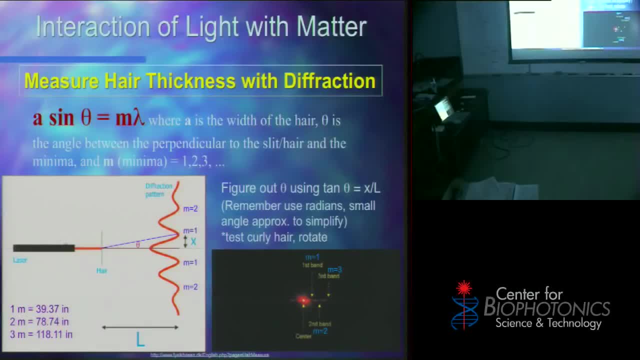 and collect your data. Collect your data. If you want to take more, you want to use your own white paper, it doesn't matter. okay, But remember that you're going to, you're going to be utilizing this data. It's much easier. 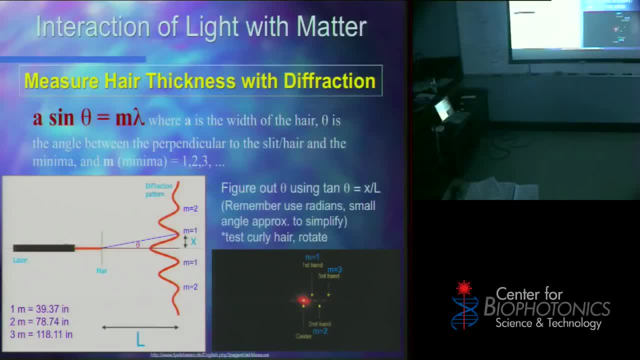 to have a piece of paper on the wall, project this on there and just draw: The first dark spot is and then the center is. Then, basically, with the ruler, draw your partners over there, cycle them and make something. Okay, It's very difficult. 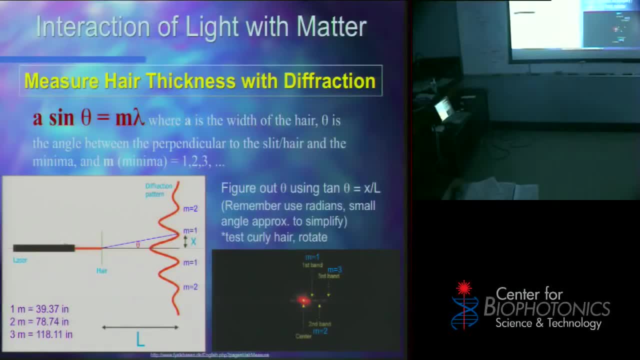 and, as you'll soon see, The last thing to do is just mark it on the paper and then later measure it. okay, Now you have to keep moving the paper if you're measuring different people's hair and you're measuring different colors. 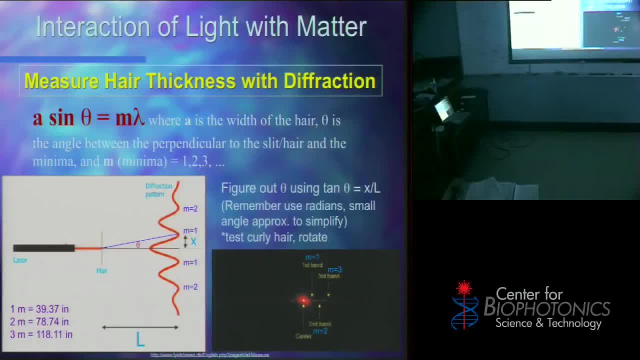 So don't get your paper up there and tape it all around. really nicely, Just keep yourself and then one piece of tape so you can quickly move it up or down a little bit and you can let other people see it. Okay, And we're going to try to. 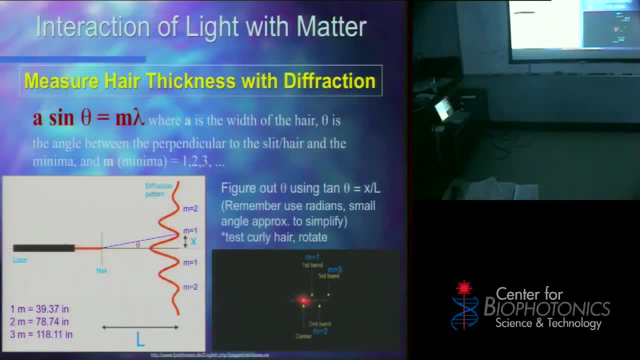 get a sense of what number is your game. You play it on the clock, okay, A little bit before that. Or if you get a number already and you want to ask me whether it makes some sense, we'll talk about it, okay. 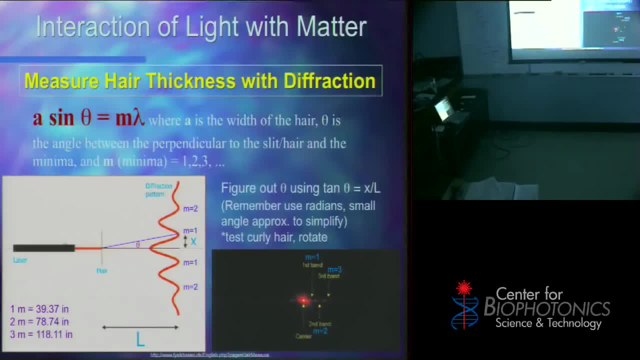 Are there any questions? Okay, Okay, And remember, you're going to be then figuring out how to represent this information and you're going to report on it, So make sure you have a good idea of how you're doing the experiment and the data that you're getting from these stuff. 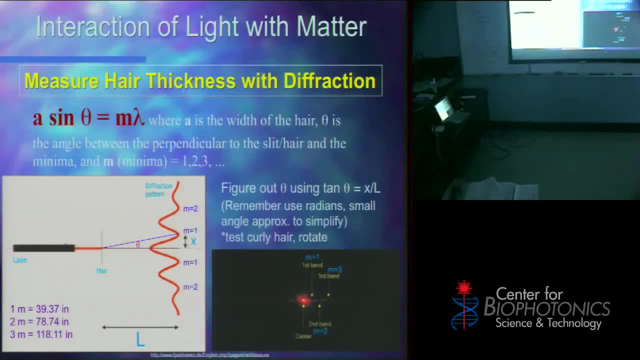 Okay, So we're going to divide up into seven groups. One group will have four people, So go ahead and divvy up and go ahead and grab your materials and start Go Again. if you're using lasers, be really careful. 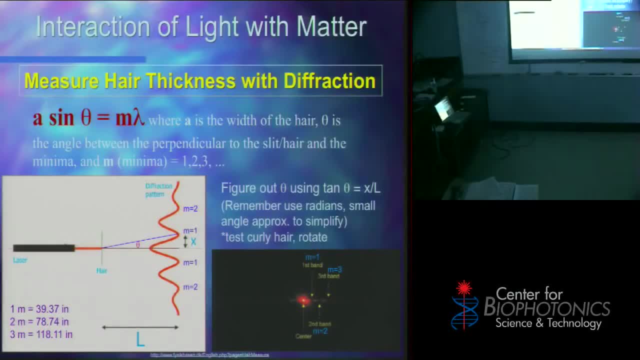 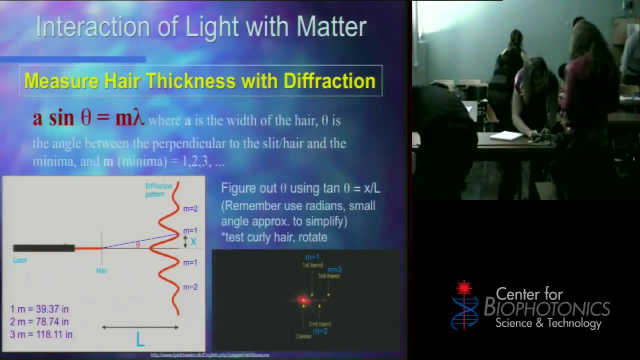 Don't try to run anyone. Don't try to run anyone's eyes. Okay, Be very, very careful. Okay, I'm just going to get another picture of you guys. Okay, I'm going to get another picture, I am. 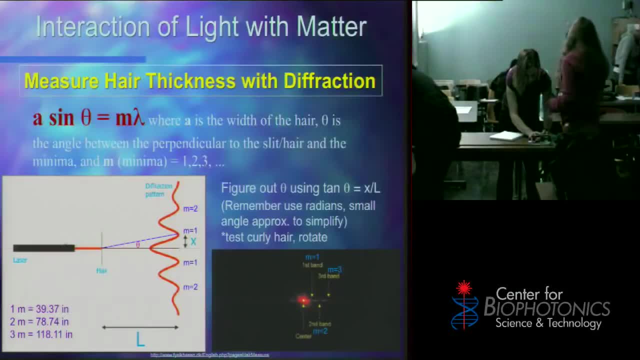 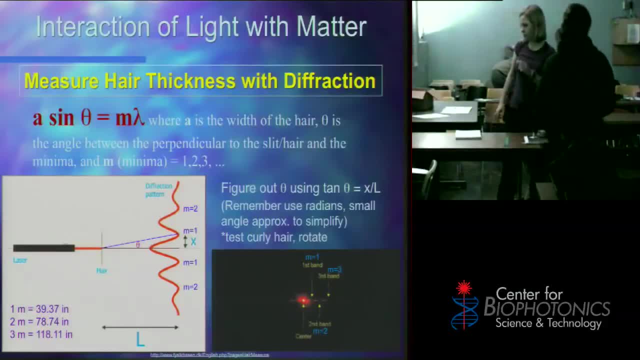 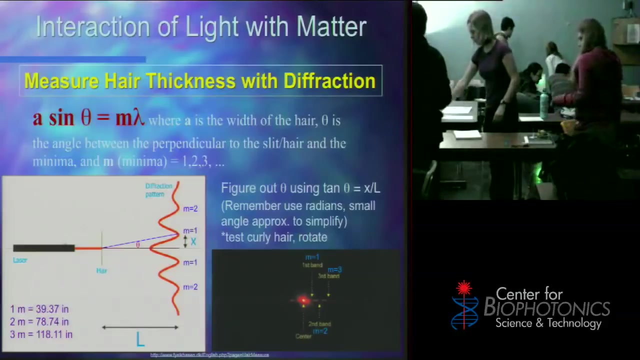 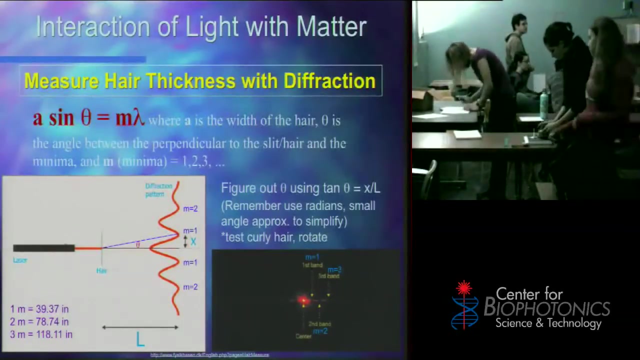 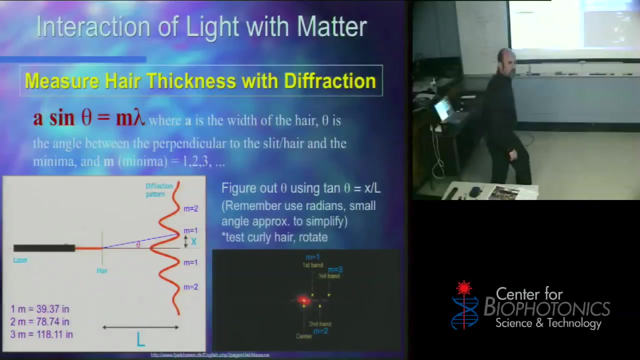 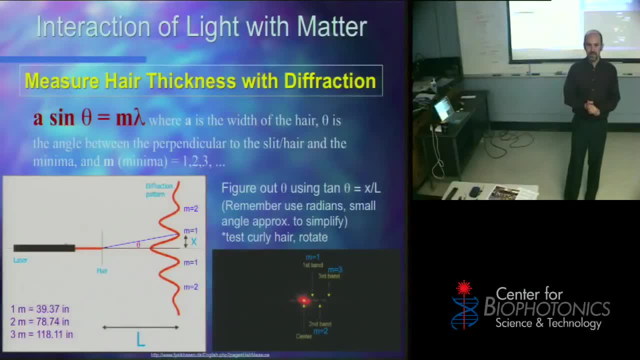 micrometers. okay, So there's a big variation in hair thickness. and remember, you guys are riding a bike up your lab reports with the data for yourself, but also the data of your classmates. I'm sorry You're using the data for yourself and the data. 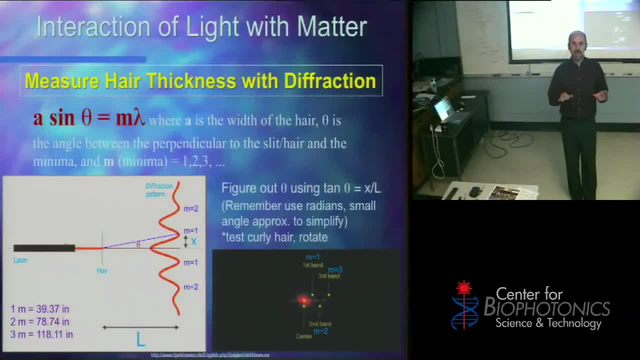 of your group mates, But you are making individual reports, So you're each making your own report, but you're using the data from the group, So we have to report on their areas as well. Yes, You will need their data, Okay. 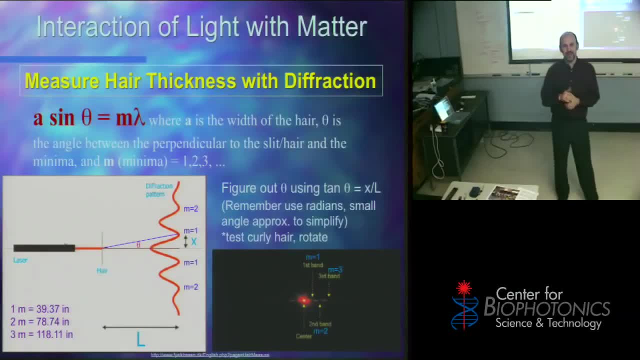 Yours is the main one, The most important, but you're also reporting how you compare with them and what their data is. That's up to you. You can either get the raw data or it's up to you. On Wednesday, you're going to be. 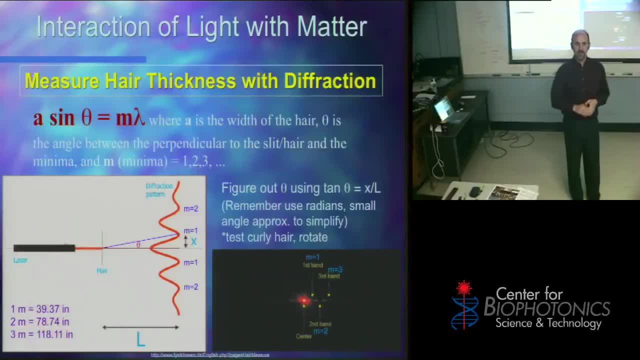 turning in four copies of the report. Okay, Because what's going to happen is we're going to block out the name on top and we're going to pass it out to three other reviewers. So we're going to review one copy and three of your peers are going to review. 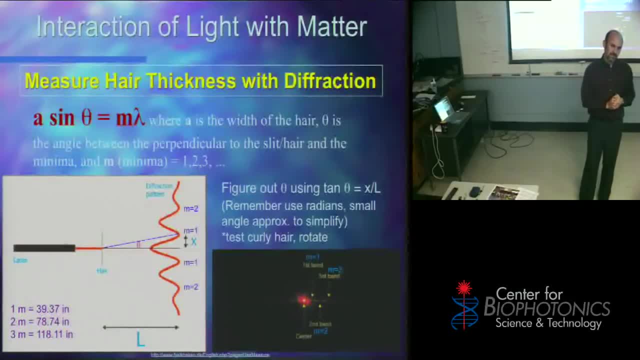 Yes, If we're turning in four copies, should we just turn in one copy with the name and the other three copies with no name on it? That'd be great. Yeah, I have to do that, Except we still need to know who it is. 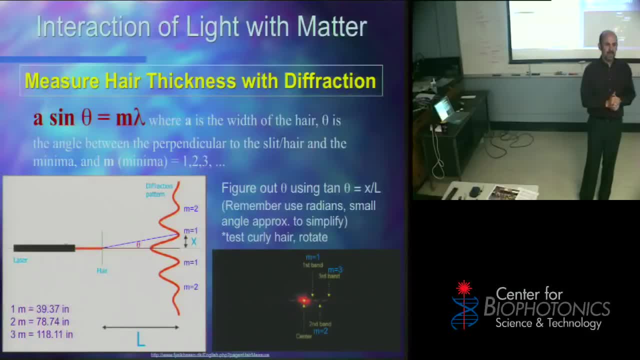 Well, if we have one copy with the name on it, That's true, That'll work. One copy with the name and three copies with no names, That'll work. Good thought, Yes, In general, when talking about, can I say: 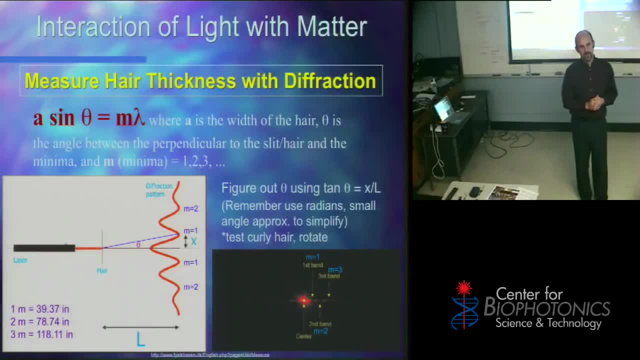 that you talked about it. The best way to do it would be to give the subject a number, So subject one or subject A, subject B, subject C. Now, in the directions that I sent out to you, it says that in your title piece you: 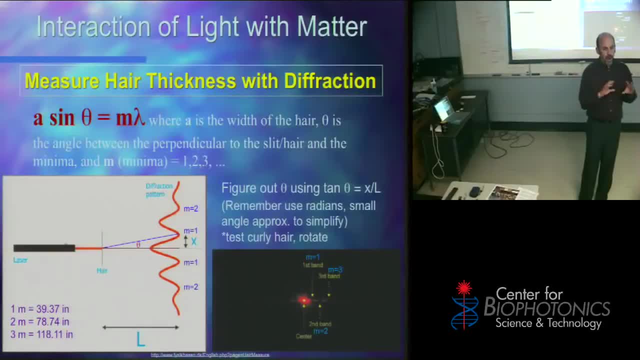 talk about who your lab partners were, And you could have a little if you wanted to. you could have a code, a key that says subject A is such and such, subject B is such and such. Except if you do that, well, people are going to know. 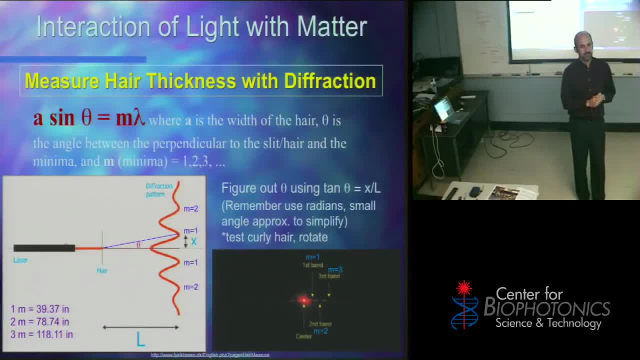 who your report is anyway. So it's okay. No, that's okay. You don't have to do that. You just say subject A, B and C. It's up to you. Whatever makes it easier for you. How does the wavelength of the laser? 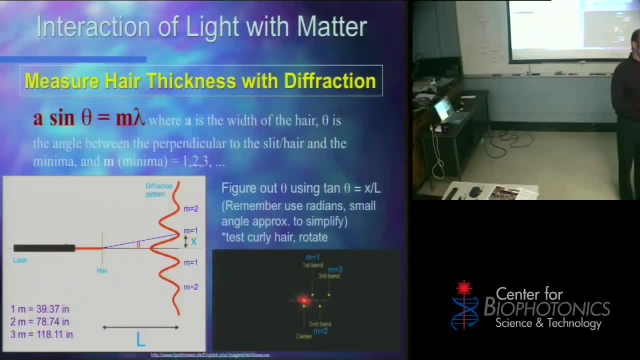 between red and green figure into this. Well, so does your hair change thickness? So this is a way to get another measurement. So do you take the average of the two? Well, you've got to think about how the error propagates. 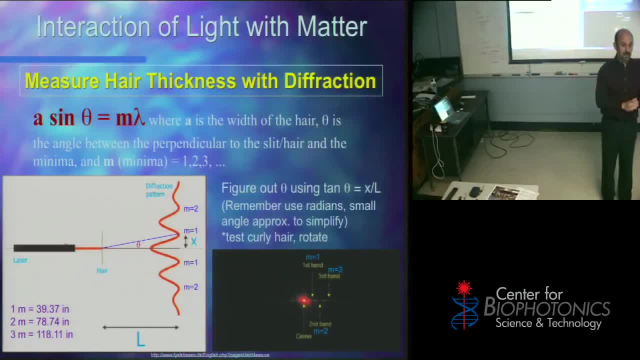 Because one of them gave you a broader separation than the other. So you have to think about that, take it into account, But that is a perfectly reasonable thing to do. That's how you want to do it. You can also average multiple readings that you might have taken. 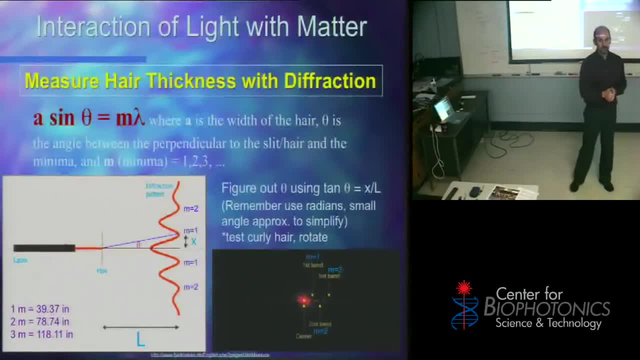 if you took more than one reading of the same hair with the same color, Okay, And what we'll try to do? after we've gotten all your reports, we'll try to do a class graph of everyone's thickness- hair thickness- But that will be separate, Don't worry about having to do that. 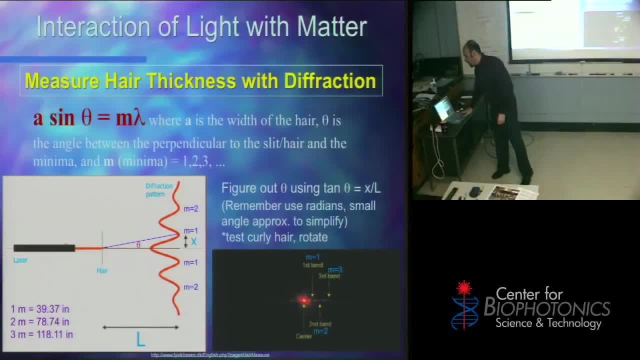 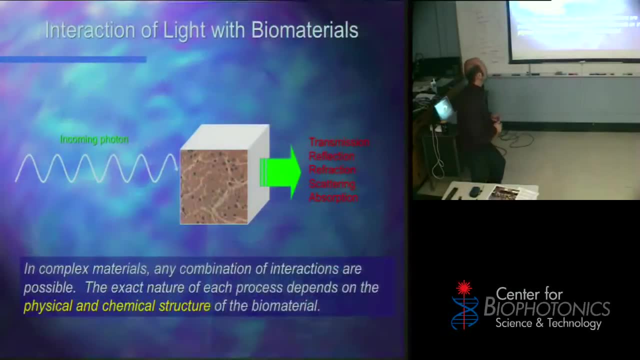 Okay, Okay. So if you have any other questions, feel free to email myself or Professor Shackleford and we'll tell you more. Okay, So let's move on Interaction of light with biomaterials We talked about last time that we can have. 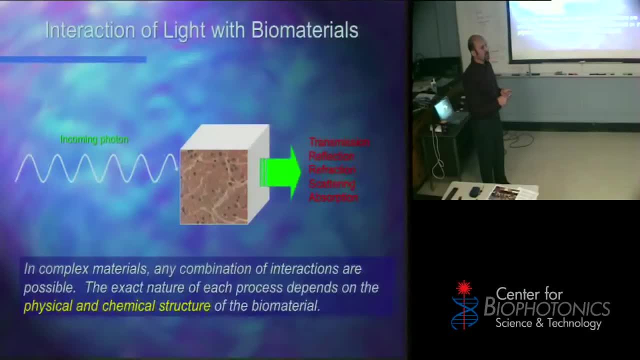 transmission, which is the light that's going through the biomaterial Reflection Refraction. What was refraction? Angle changes. Basically, the photons slow down when they get into something of higher density. They just slow down And depending on the angle at which they're interacting with that surface, 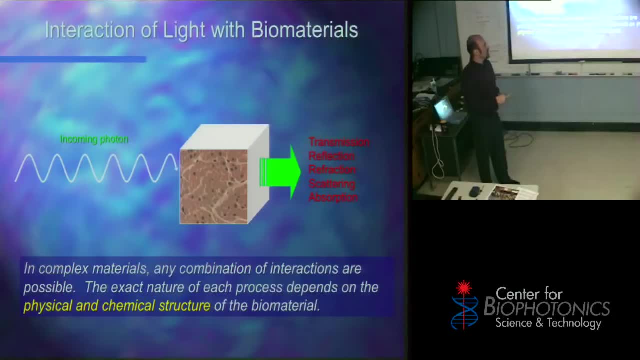 they will bend further. Okay. Scattering and absorption: Okay. So the exact amount or how these things work out in the material was going to depend on the physical and chemical structure of the biomaterial you're interacting with. Okay So, 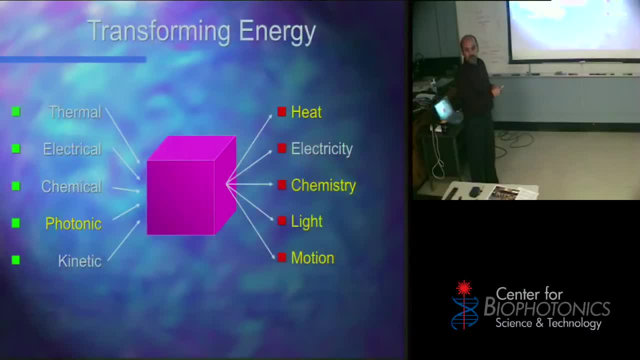 you can have photons interacting with the matter and they can cause heat. You can heat something up by having the light interact with it. Can you give me an example that you guys feel, hopefully, on a regular basis? Sun Makes you feel warm. 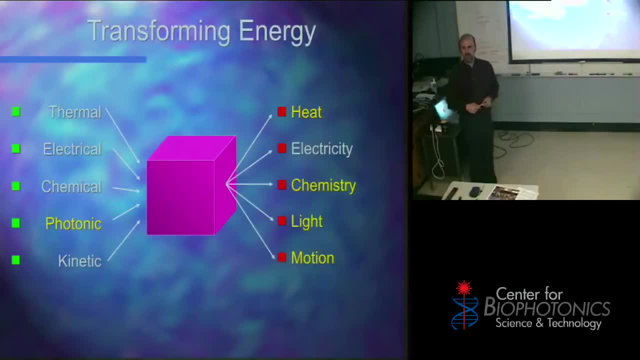 Okay, You can have photons going in causing chemistry to happen. What might that be? What do I mean when I say chemistry to happen? Yes, Yes, So they actually make a chemical reaction happen. I can break bonds, Remember. 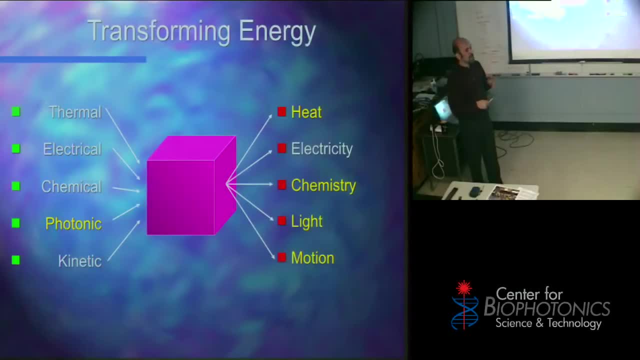 I can cause molecules to get excited, But that usually corresponds to heat. When it's chemistry, it's either usually a conformational change or a bond breakage, things of that nature. I can cause light, I can put light in and I get light out, And we know. 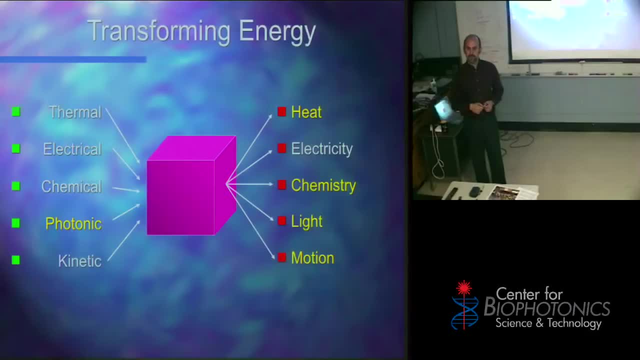 that that can happen by just straight transmission. How else might that happen? Yes, Fluorescence, Yep, Fluorescence, phosphorescence, Perfect. And I can cause motion. What might I mean by that? Back there, I'm just saying: 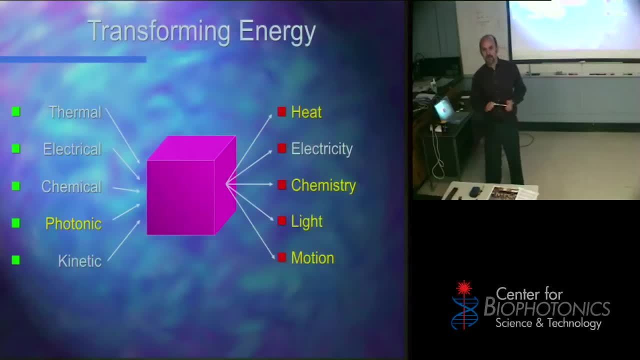 on Monday I'm going to be on a date, Chris, Use highly concentrated lasers to push a cell down. Yeah, I can actually travel a cell. Can you use a microwave to use the molecules? You can think of it if you want to think of it. 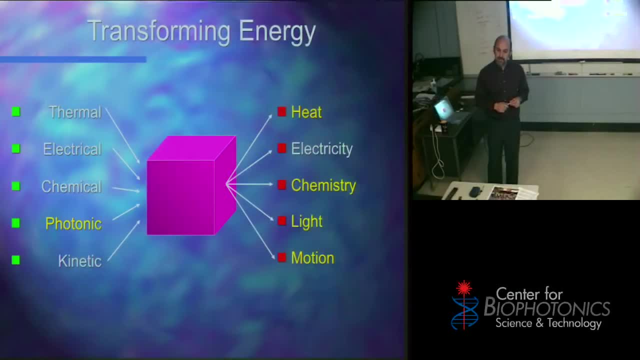 as motion within the molecules. that's fine too. Yeah, the rotations: Yeah, that's another good point. Okay, So photonic energy can come into a system and it can cause all kinds of other things to happen. Now we can do electricity too. 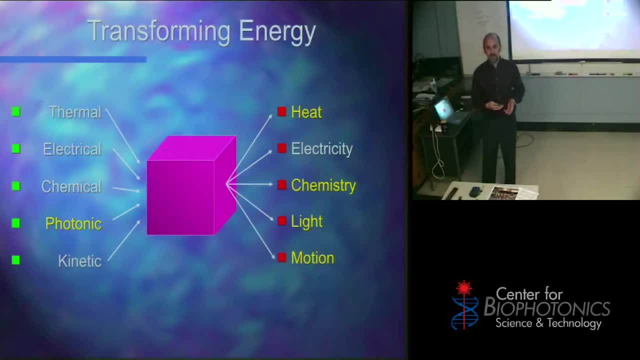 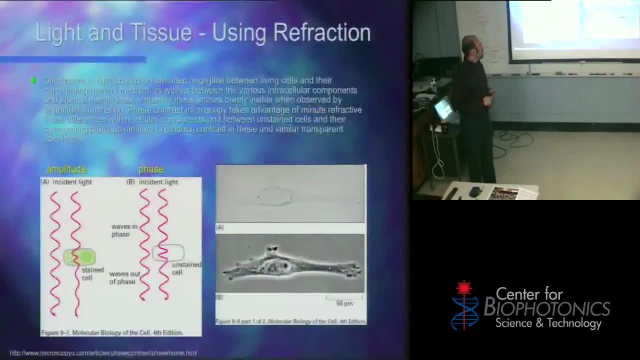 Solar panels, But it's not something that tends to happen in living tissue- Okay, That's why I'm not highlighting it. So I'm going to talk to you about some ways in which we can use these properties. So the first one I'm going to look at is refraction. 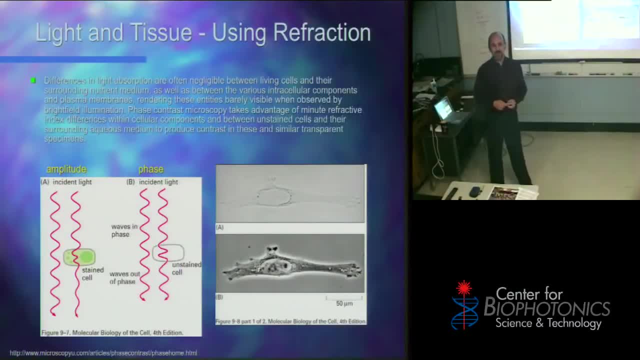 Whenever we do microscopy, when we look at things under a microscope, the main object is to see something under the microscope and to see it really clearly. That's why we use the microscope Right. We want to learn about something really small. To do that, we need to be able to see it well. 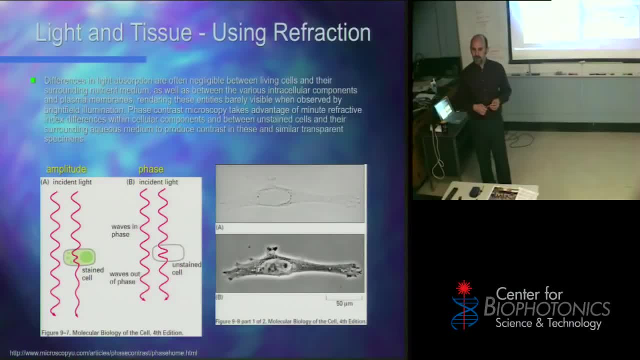 And how many of you have used the microscope before and you put in some pond water or something and things look very dull. Has that ever happened to you? Very plain, There's not much there. Well, you can get something like this in an aneba here. 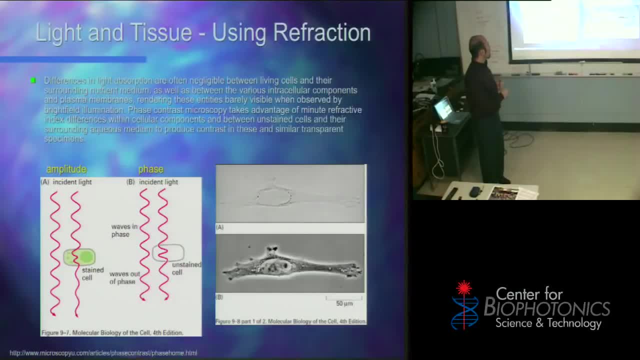 We can use techniques to take advantage of the light being slowed down inside of a cell to give us contrast in an image. So this is a type of microscopy that allows me to get an image that looks more like this, Taking it advantage of the fact by using some special 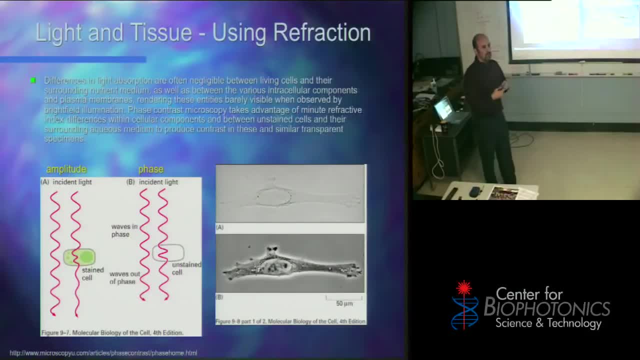 optics that it'll make contrast happen when there's a difference in the speed of the light going through the material. So I get this kind of a pattern. This kind of microscopy tends to give you this halo type of piece. It can be called phase contrast. 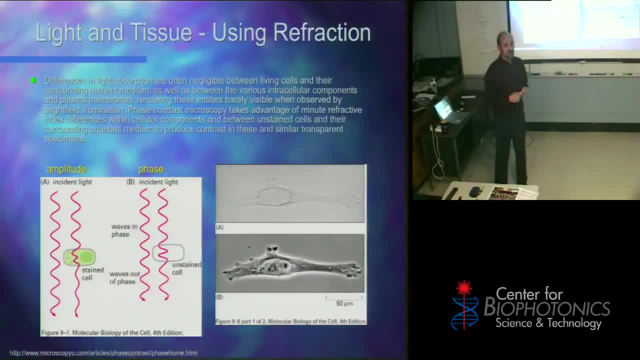 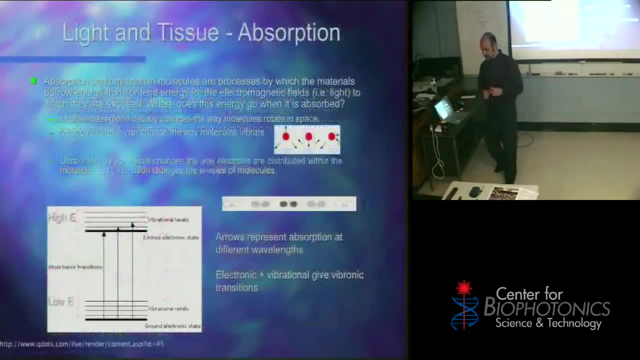 or differential image contrast. These are some different names for this type of microscopy, And you're going to be getting introduced to different types of microscopy as we go on through this course, especially when we talk about tools. We talked the other day about absorption. 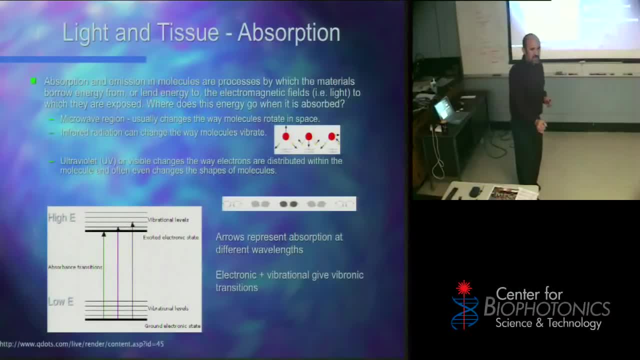 So absorption photons come in. that energy excites an electron to a higher energy level and that can manifest itself in different ways. If microwaves are absorbed, it usually changes the way molecules rotate in space. This is what you were talking about. 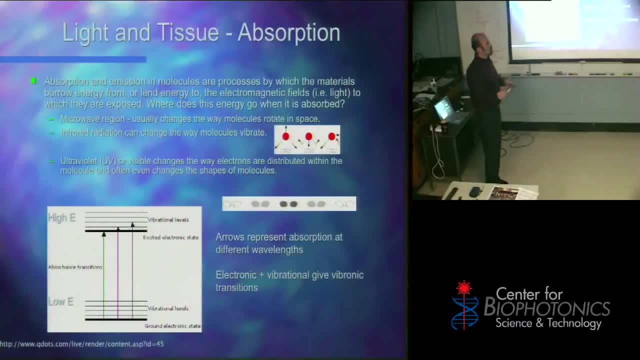 a few minutes ago. If we bring in infrared radiation with living things, usually they cause a change in vibration. Okay, Rotation and vibration can both lead to the perception of heat, What we call heat In infrared radiation. that makes a lot of sense. 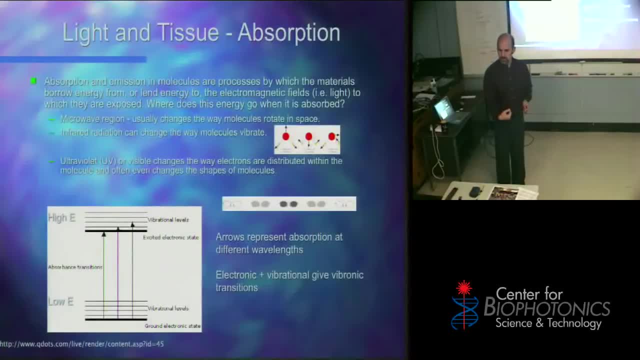 Ultraviolet or visible photons. when they're absorbed, are they higher energy or lower energy than the infrared? Higher, Okay, And even higher than the microwaves- Okay. Microwaves are the lowest. Those will change the way electrons are distributed within a molecule, and it will. 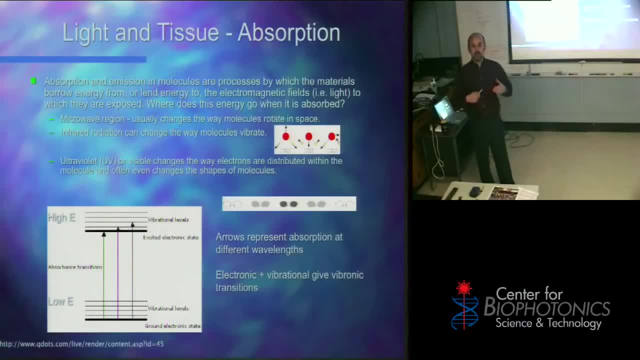 often change the shape of the molecule or potentially even break the molecule. These are those sunglasses that when you go outside, they will change color. Well, guess how those work? They take in the high energy light that you're getting from the sun. 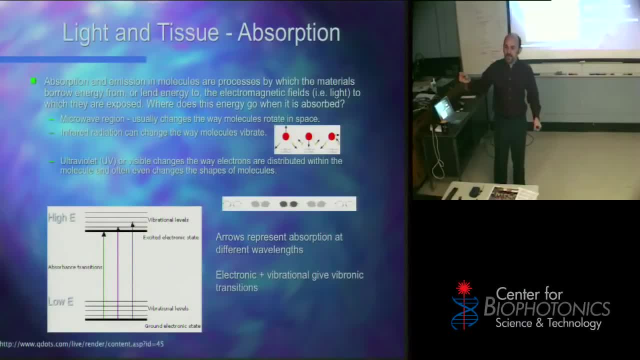 or from any kind of bright surface and that causes a conformational change in the molecule. That conformational change in the molecule causes them to darken and it's reversible If that energy goes away and that absorption isn't taking place. 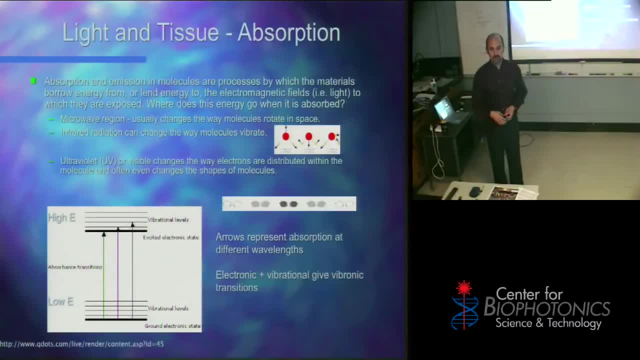 the molecules go back to their natural state and it becomes clear again: Yes, How come after one time of this factor they don't change as much and they don't go all the way through? Okay, That's basically because these reactions are all, for the most part. 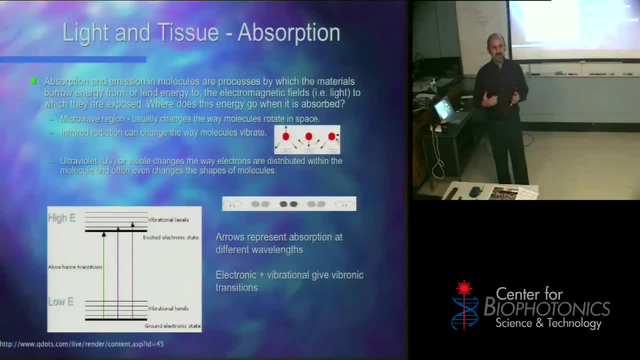 reversible, But over time, some of those structures change in such a way that they can't reverse very easily, Are they? Some of them? Some of them? Some of them basically get stuck. Okay, So you can imagine over time as more and more get stuck. 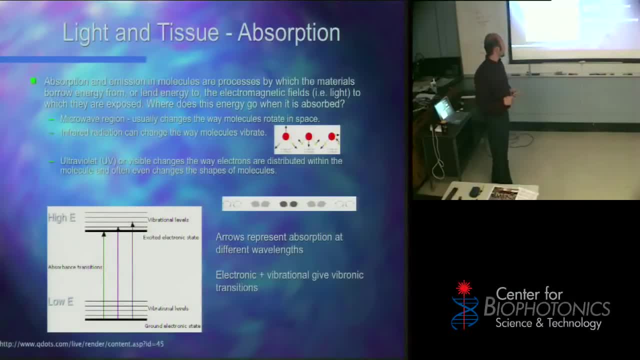 the change isn't as great anymore. Okay, Now usually everything's happening at the same time, So if I have a energy state change that's caused to like ultraviolet or visible, I get an electron-jumping energy level. 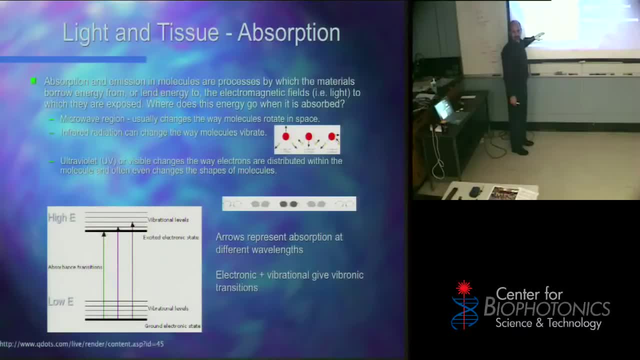 When we make these other lines like this: these are vibrational levels, Okay, And changes within these lines would be changes in vibration in rotational state. And if I were to make even more lines in between these lines, if I were to make little lines like this: 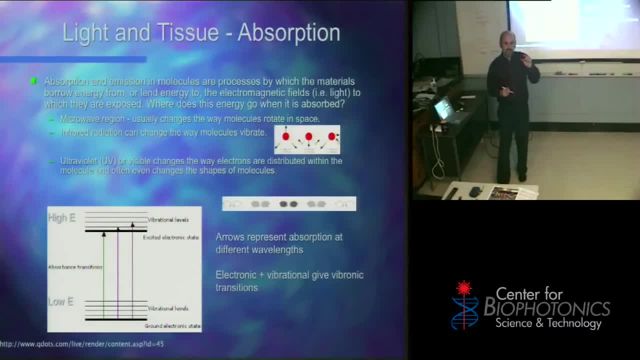 little line, little line, little line. those would be representation of the energy change in rotational states. So usually when I jump and I absorb energy, I'm absorbing energy and I'm changing electronic state, which is the high energy state. 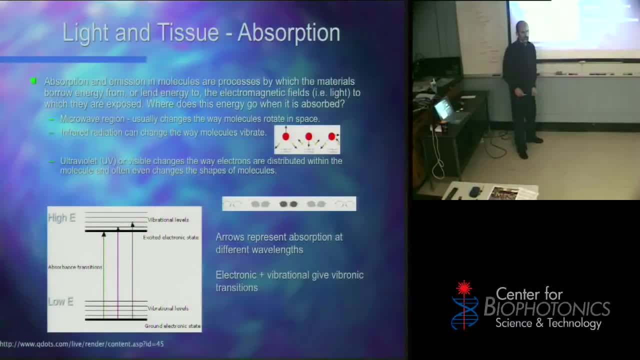 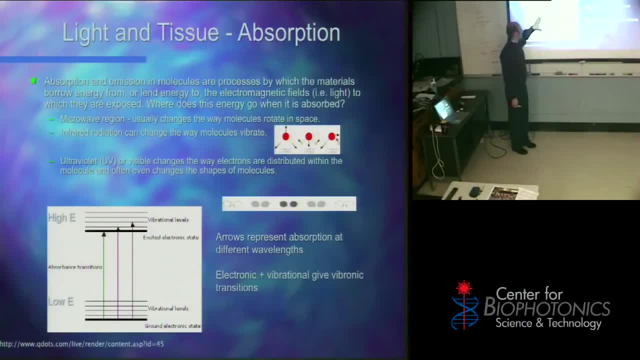 with the energy I'm bringing in, Because the molecule that I'm working with can only absorb energy if there's a specific jump it can jump to. If there isn't a jump that corresponds to an electronic, vibrational and rotational state, it can't go there. 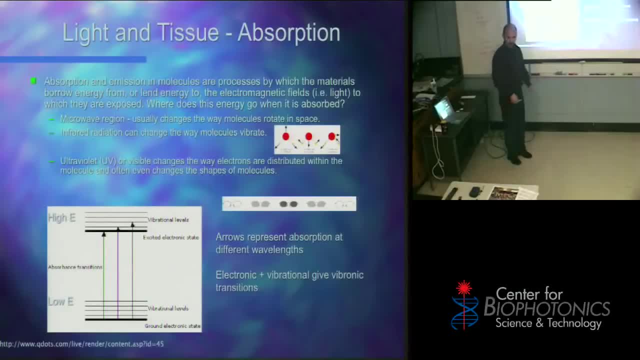 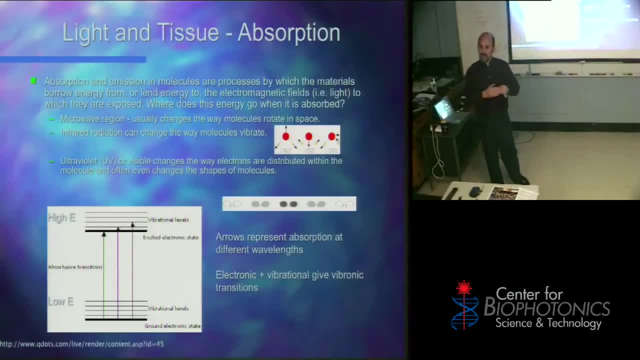 Okay, Okay, Okay, Okay, Okay, Okay. And then you can get relaxation through rotations, vibrations and electronic jumps. Now that sounds a bit confusing. You'll be hearing a little bit more about it as we keep going. So, electronic versus vibrational. 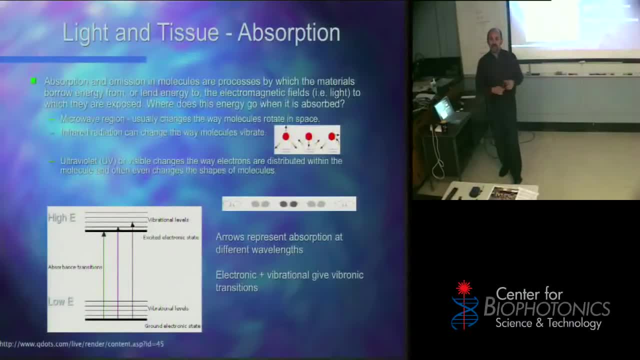 sometimes they call them vibronic. They're just different names. But when you have these transitions you're changing usually electronic state, vibrational state and rotational state, And primarily we only talk about the rotational and vibrational. I'm sorry. 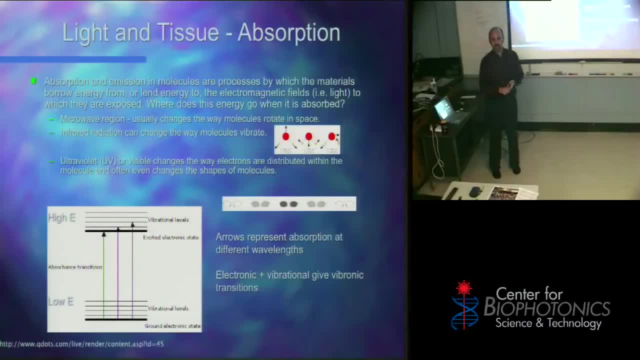 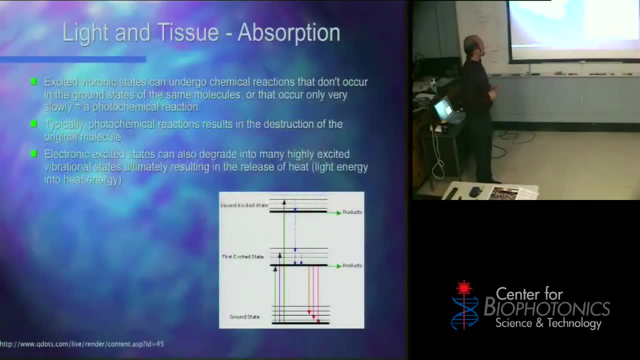 We're going to talk about the vibrational and electronic. We don't tend to talk about the rotational because it tends to be such weak energy, Energy changes. So when we're working with light and tissue, these vibronic states, these jumps in energy, 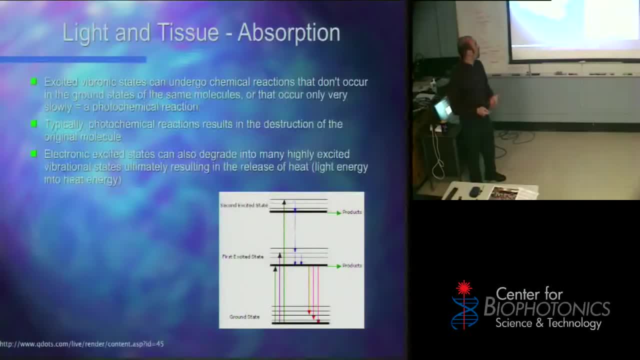 can basically cause chemical reactions to happen that don't normally happen. Okay, So photochemical reactions result in the destruction of the original molecule, So in most cases things are not reversible like what I was telling you before. When you have the light interacting, 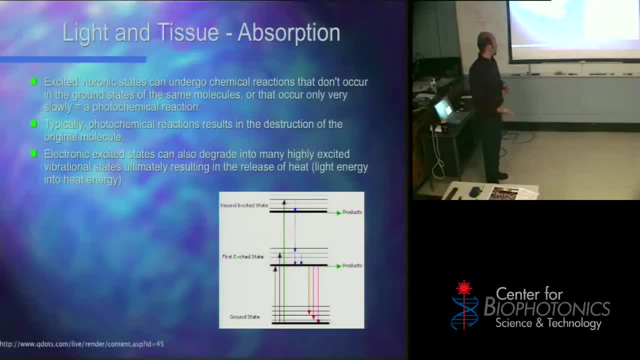 it's absorbed and it causes something else to happen. It causes some other products to be created. You can also basically have an absorption of a photon, and there's so many different ways in which those photons relax that you get a release of heat. So, absorption of photons. 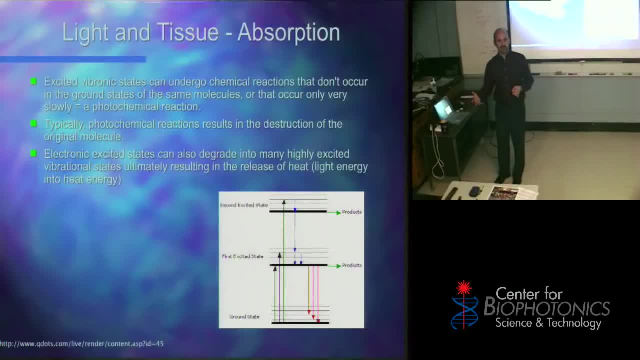 often releases in some kind of heat and other things. So it can result in the heat, it can result in the conformational change, it can result in the molecular change and all those things can happen simultaneously And when we want to destroy. 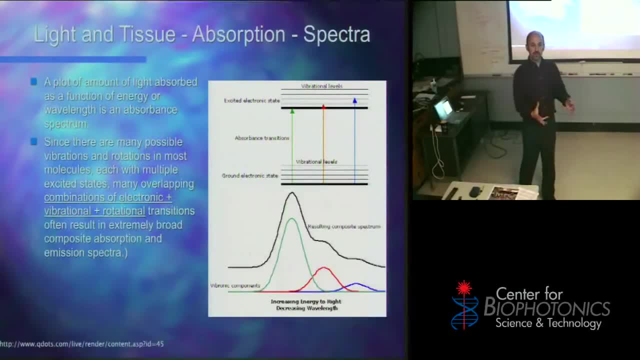 describe how a certain molecule, sets of molecules, are absorbing light. we create something called a spectrum And that spectrum tells us, shows us energy in one axis and it shows us the amount of that energy that was absorbed. Okay, So we get an absorption spectrum. 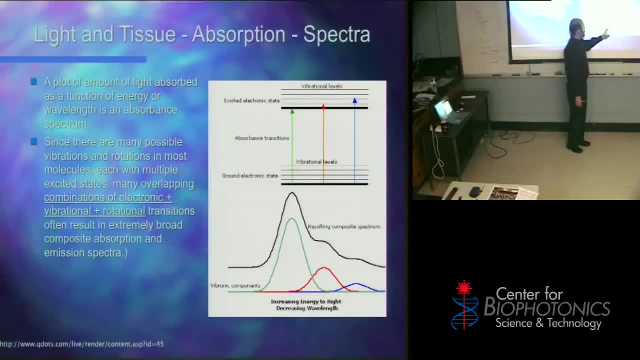 that says this wavelength was absorbed a little bit, this wavelength was absorbed a lot more, this wavelength was absorbed the most, this one less, this one less, this one more. and it tells us- And by the shape that we get, we actually can see: 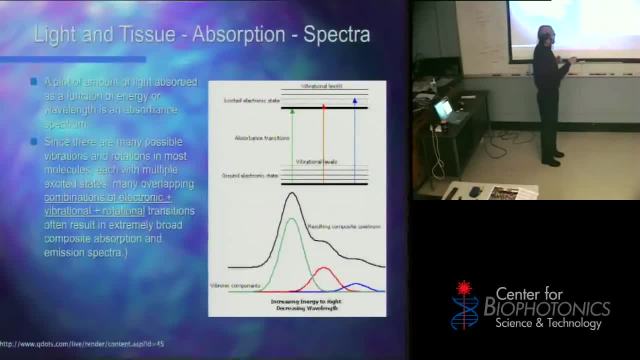 for example, this is showing you. this green transition here would correspond to this, the red transition would correspond to that and the blue transition would correspond to that. And when you actually see the spectrum, it would look like this. It would look like these blobs: 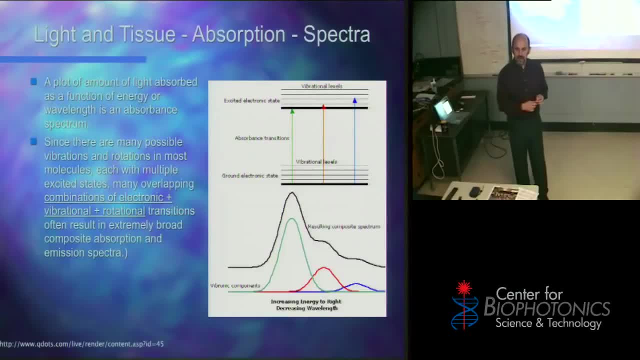 So in a spectrum you can see that the spectrum is a spectrum. So in a spectrum you can see that the spectrum is a spectrum. You can see the various ways in which energy has been, in which electrons have been absorbed to go into different electronic. 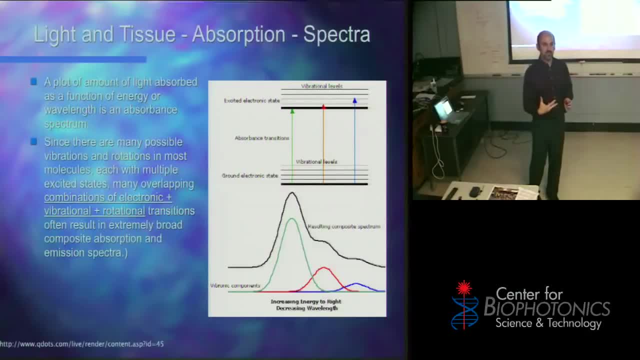 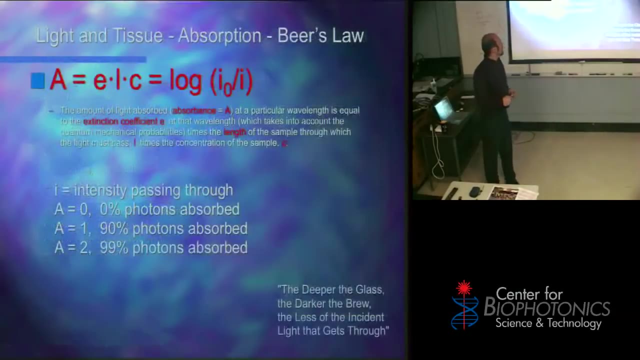 and vibrational states and rotational states. That's what the spectrum shows you. It shows you where those absorptions took place, at what energies. Okay, That's how we learn this, That's how we figure this out And the way we characterize absorption. 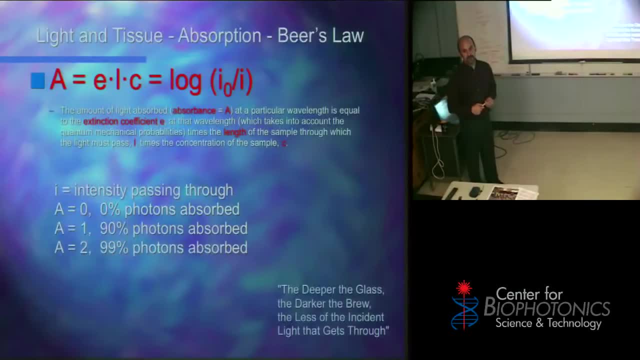 is by a formula known as Beer's Law. And Beer's Law, the way people remember it is: the deeper the glass, the darker the brew, the less of the incident light that gets through. Okay, That's a little shortcut for remembering. 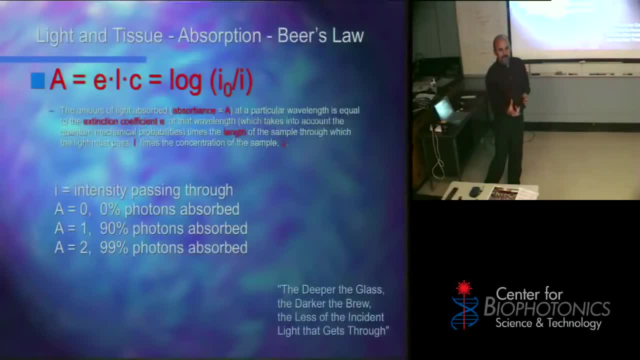 But it basically says: I can quantify the amount of light that is absorbed. And I can do that and it's very specific to a given molecule or a given combination of molecules. The absorption is equal to the extinction coefficient at a certain wavelength. 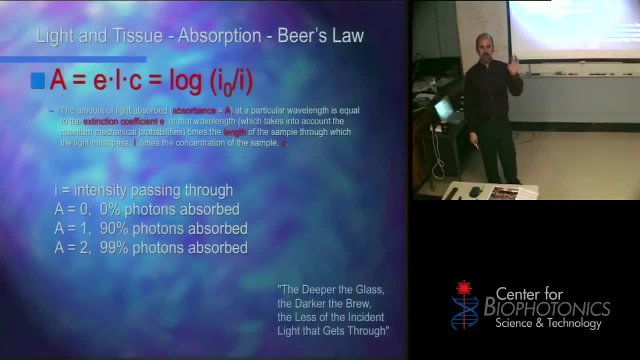 So what this says is for a specific molecule. I have this very specific number at this specific wavelength, So DNA will absorb at 250 nanometers. this much It's very specific. Then I multiply it times the path length of how much of my molecule. 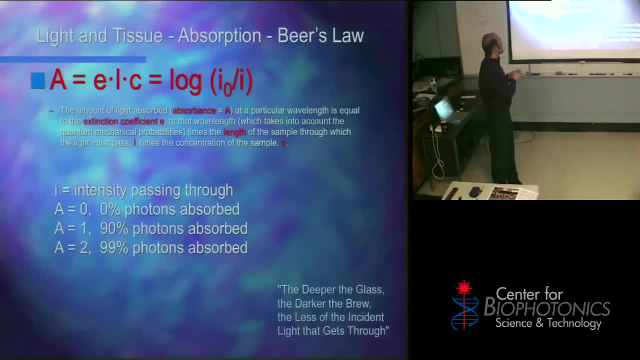 I have the light going through times the concentration of my molecule, So you can imagine the absorption increases. if I double my concentration of the absorption, My absorption doubles. If I double the amount of length that I'm passing my light through, my absorption doubles. 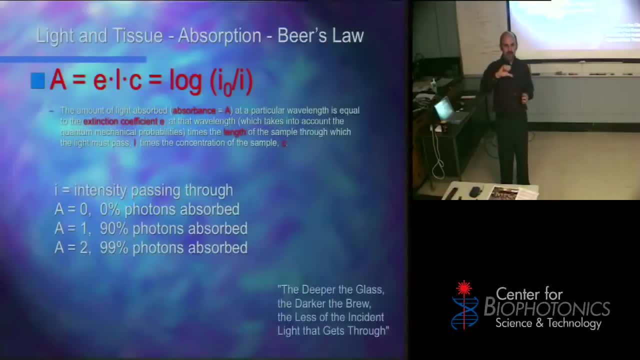 Okay. So it kind of makes sense If you were to take some food coloring and put it inside a little test tube. if you put twice as much of the food coloring in the water, not as much light would get through. Okay, Okay. 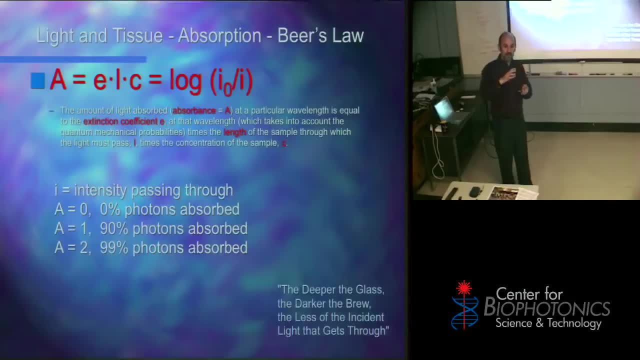 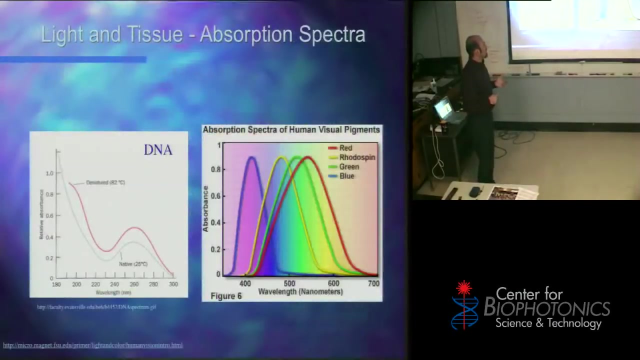 If you were to take a bigger tube with the same amount of water to food coloring mixed together, not as much light would get through because it's a thicker piece going through. Okay, Does that make any sense? And when we look at specific living tissue? 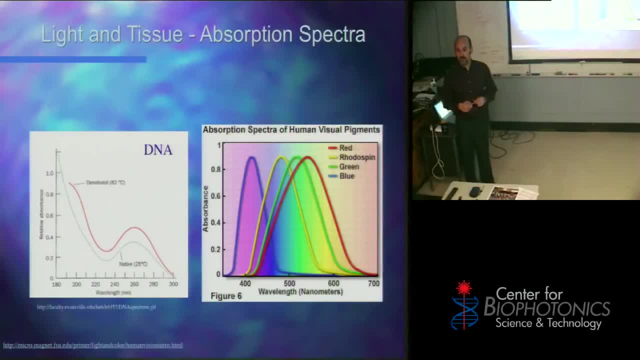 and we look at their spectra, okay, which shows us how light is absorbed by them. if we look at DNA, we can find out something about the DNA. Here's the wavelength, the 180 nanometers. this is all in the ultraviolet. 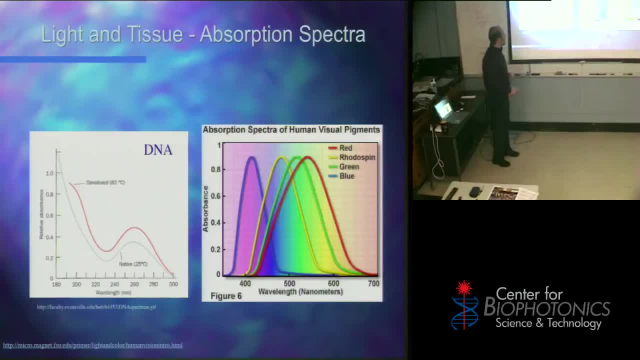 up to 300 nanometers. Okay, We can see that DNA that's double-stranded, native, will have a spectrum that looks like this: DNA that's denatured, meaning that it's fallen apart, the two strands are not together anymore. 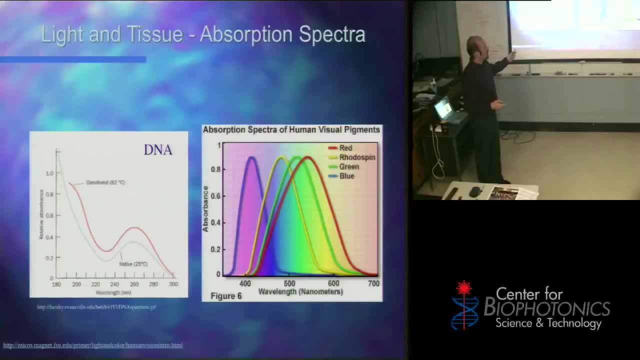 will look like that DNA at 82 centigrade will separate. At 25 centigrade it tends to be together in a double helix, Okay, And you can use this to figure out properties of how strong those helices stick to each other. 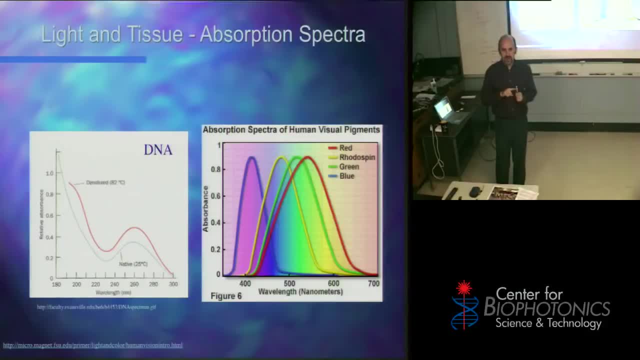 I spent my first year in graduate school doing that. I created little structures called hairpins, where you would make a piece of DNA or RNA that would be single-stranded, make a loop and then attach to itself again, And what I would do is: 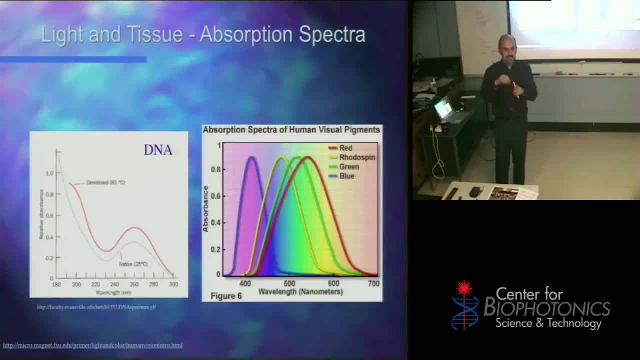 I would work for two months to get my sample and then I'd stick it inside a spectrophotometer and I'd heat it up while I measure. and I measured at 254 or 260 wavelengths around this region And I saw it change. 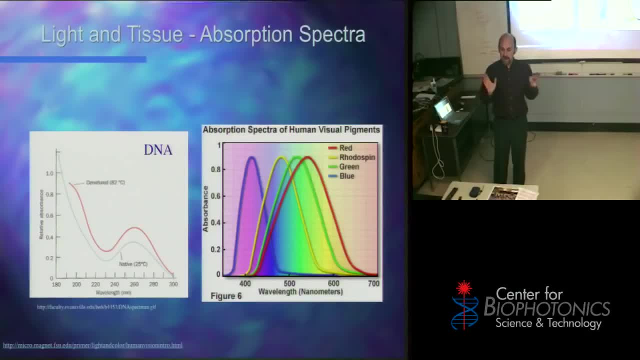 and I could tell exactly how much energy was involved in making those bonds in the hairpin Or whether even the hairpin was made Okay. So you can tell what's happening: changes in conformation based on looking at the spectrum Now in your eyes. 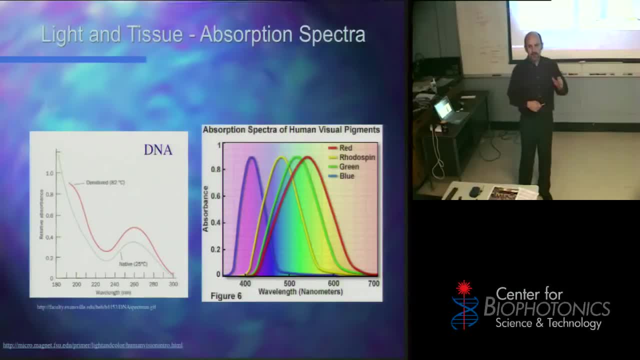 you have four pigments that absorb light, And depending on how much each one of them absorbs is where we get the idea of what color we're seeing. So you have one that absorbs blue, and this is its absorption spectrum: Rhodopsin. 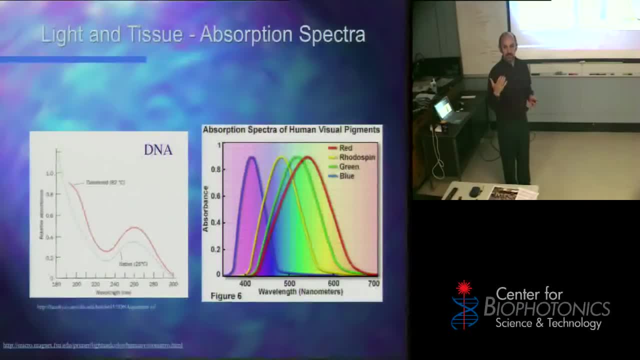 that's the one we tend to use at night, that we just sense it absorbing just as seeing light or not light. Then we have a green one and a red one, And depending on how much each one of these pigments absorbs, 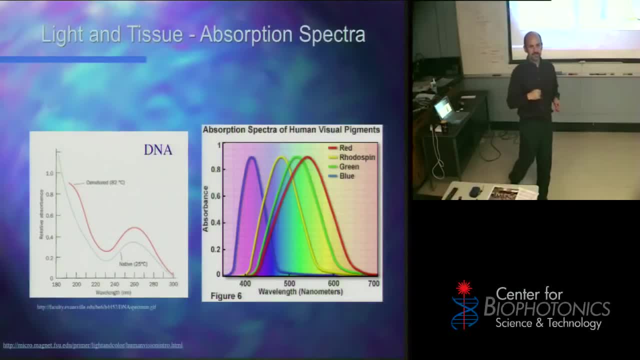 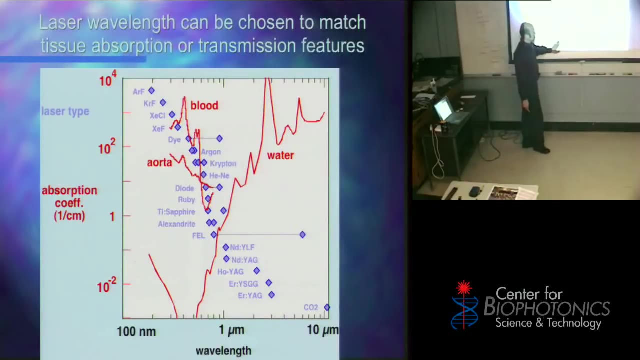 we, our brain, interprets the color. Okay, These are their absorption spectrum And the other. the last thing I want to tell you about absorption in living things. this is a wavelength: 100 nanometers. this is the equivalent of one micrometer. 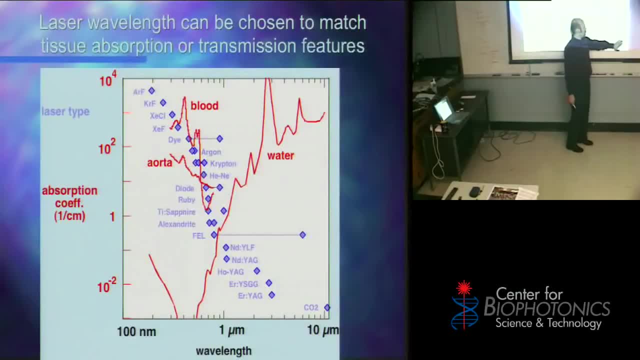 or a thousand nanometers. This is 10,000 nanometers. We have what we call an optical window for living tissue, And what this says is: this is the spectrum of blood. This is how blood absorbs At those wavelengths. This is how your aorta absorbs. 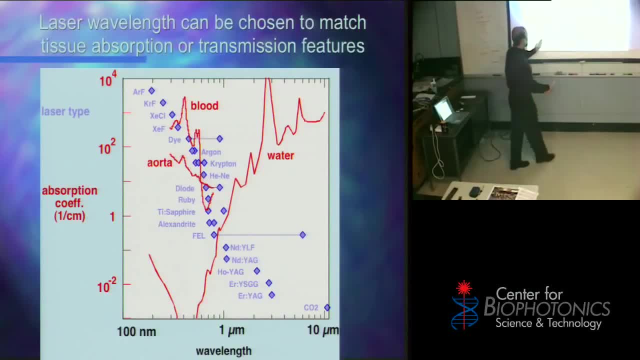 This is how. where water absorbs, So wherever water has a very low absorption in this region, from here to here- is where we have a good opportunity to study living things directly in living things, So we can utilize the fact that there's not a lot of absorption in this region by water. 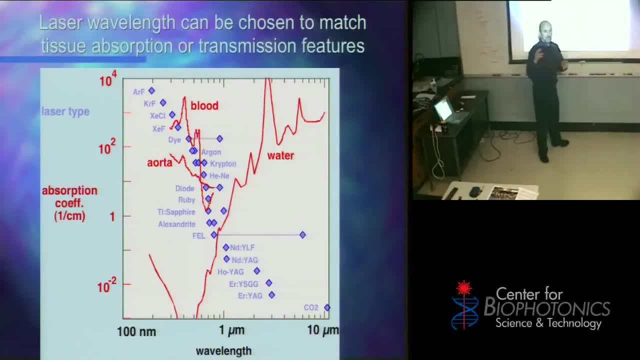 and we can utilize the fact of this blood spectrum to figure out your amount of oxygen in your blood. Okay, With that little tool that we made. Okay, So we have a window that tends to be this would be 200,. 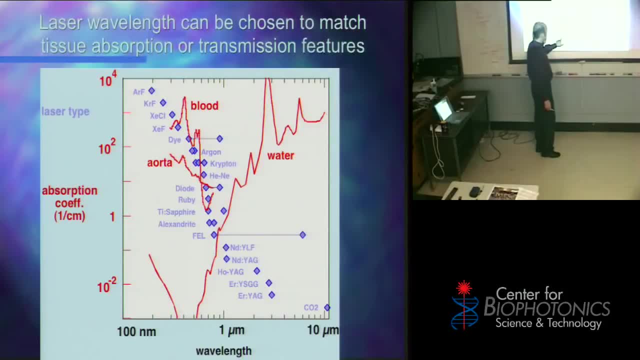 300, from about 300,, actually from about 200 nanometers- 3,, 4,, 5,, 6,, 7,, 8,, 9, to about 900 nanometers, where the absorption of water is relatively low. 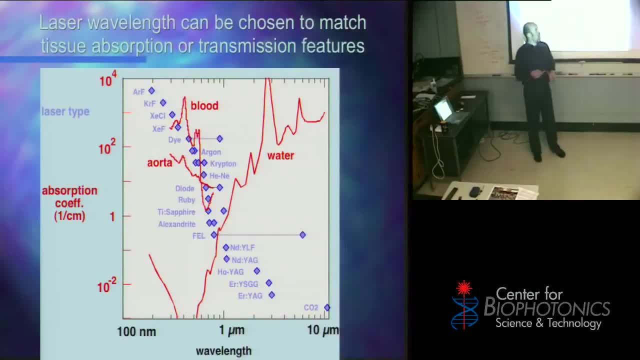 This is a log scale. It's relatively low, and so we can see other things just based on how they absorb light. Okay, Once we get out here, into this region, over here, basically, where things like this absorb less than water, 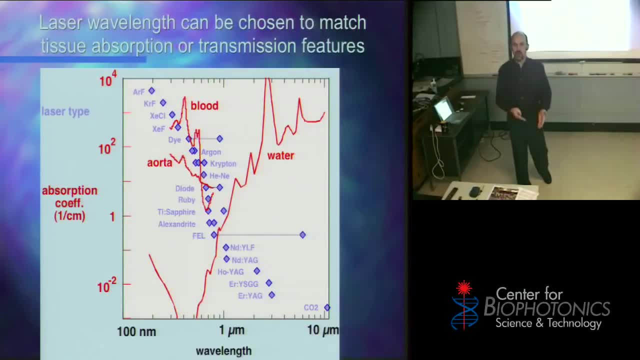 then we can't use those wavelengths very easily, because water is always the main thing that we're seeing in something alive And it blocks us from using those wavelengths. Okay, So the optical window- this is another way to see it. This one has a few more things on it. 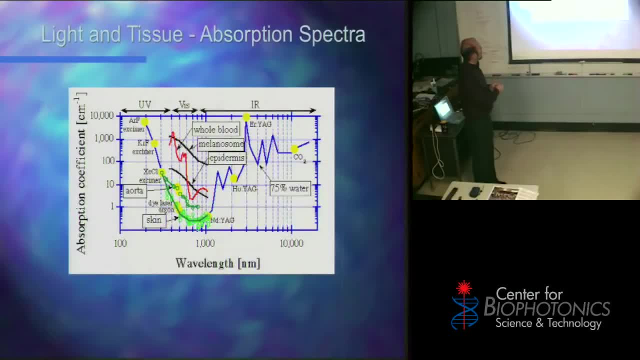 It has whole blood epidermis. it shows you the aorta, it shows you the absorption of skin, it shows you all these different things and these little yellow spots. it just shows you lasers that have that wavelength. So what laser would you use? 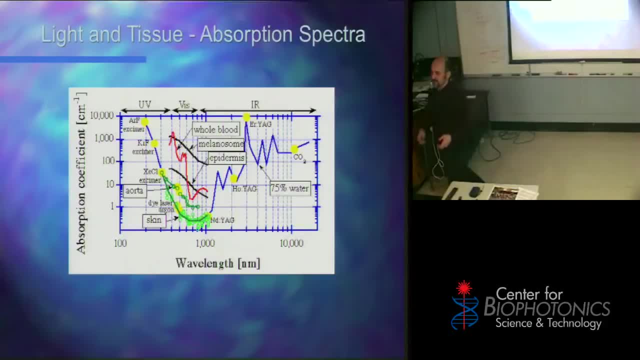 to look at what part of the spectrum? Oh, the keys. Thank you. Okay, So again, this is the optical window that we have. It tends to be from about 200 to about 1,000 nanometers. Okay, And what does it mean to be the optical window? 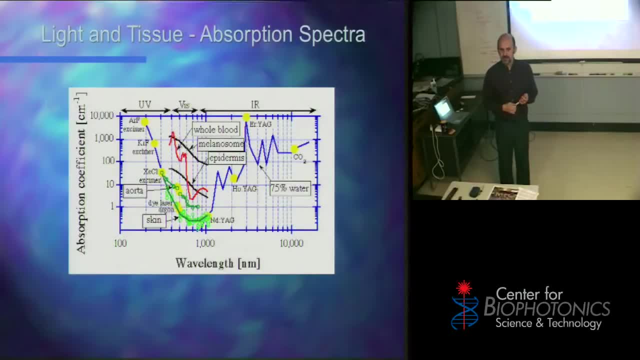 Why do we call it that? Why is it relevant to us? Yes, Yes, Basically, water is not dominant in that region. Okay, The absorption of water is not dominant, So we can look at the absorption of other specific things inside the tissue. 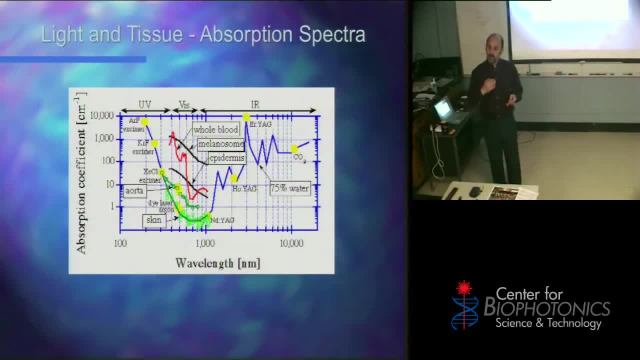 The DNA, the RNA, certain proteins, the blood, the hemoglobin. We can look at all those things in that region just by using light. in something alive, Okay. In the other parts of the spectrum, water overwhelms us. It's very hard to detect the signal above and beyond the signal of water. 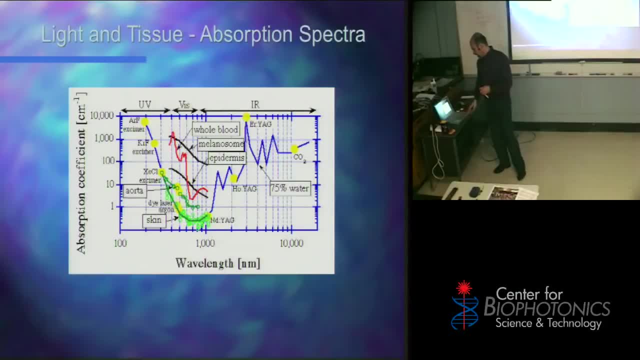 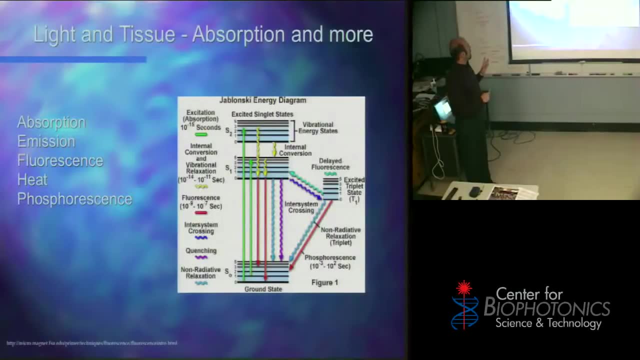 Not impossible, but very hard, Okay. And so, to kind of recap, remember: when light is absorbed you can have fluorescence. When light is absorbed, you can have heat. When light is absorbed, you can just have it be absorbed and then re-emit it right away. 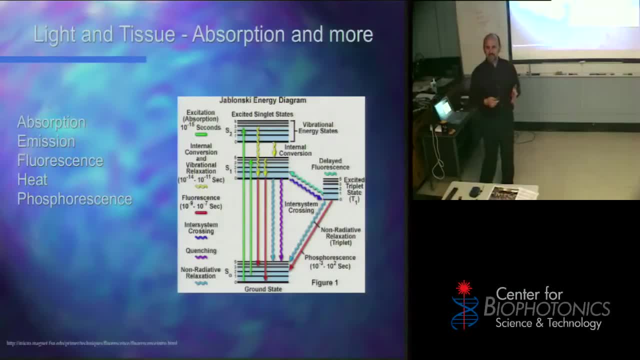 And you can also have phosphorescence. So all of these things happen simultaneously And, depending on the specific molecule, you get more or less of one over the other, And also depending on the conditions the molecule is in, what it's near. 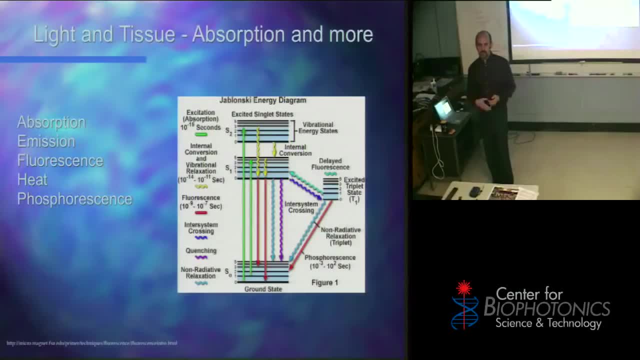 Okay, So that's how we get information about what's happening to molecules. Questions about that. So is it possible to have: if I have a set of molecules inside living tissue and I shine light and that light is absorbed, could I have fluorescence and phosphorescence happening? 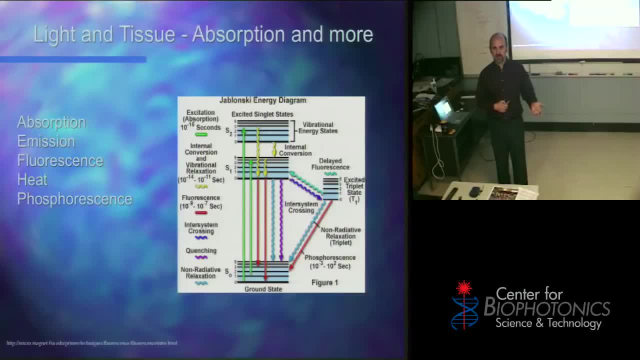 And heating. Is that possible or is that impossible? It's possible. You can have all those things happening. Are they all going to be the same amount? Okay, They're going to vary. There's going to be a. It's all a combination. 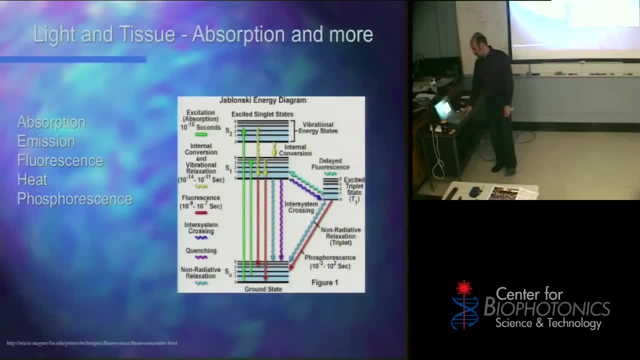 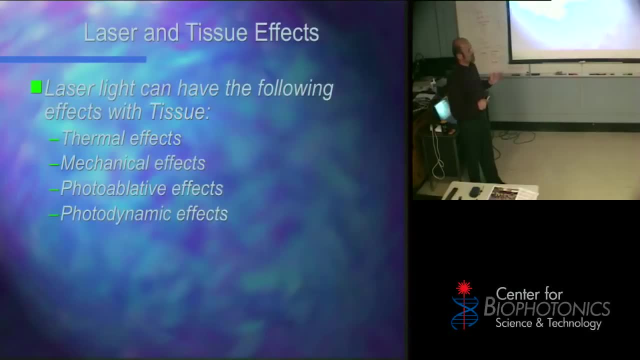 Let's pick one that we're going to look at. Sometimes we pick more than one, but usually we just pick one to look at. Okay, So let's move on now to laser and tissue effects. So laser light can have the following effects with tissue: 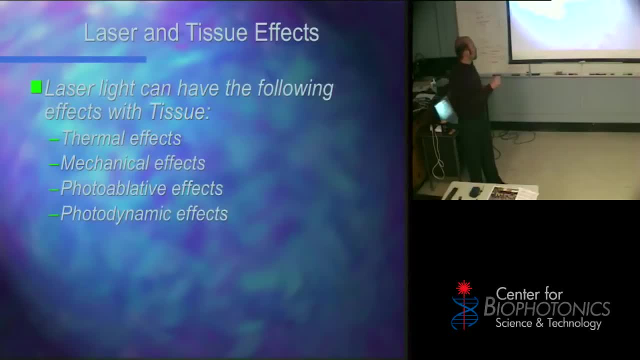 Thermal meaning heat things up. Mechanical like move something. Photoablative- Photoablative just means poof, It means I take that tissue and I make it into vapor, Make it into nothing, Okay. And photodynamic, That means I can have light being absorbed. 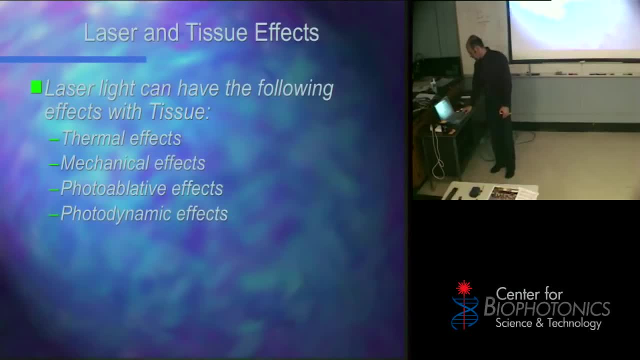 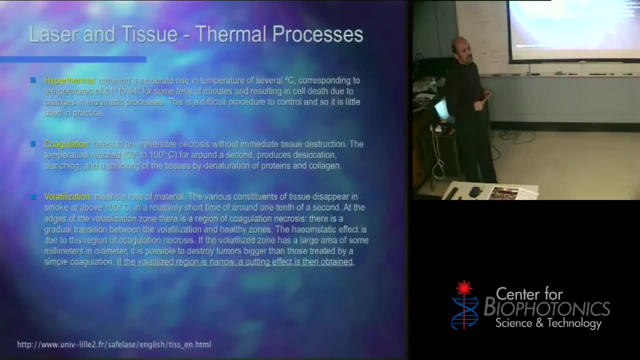 and cause some kind of chemical change that can cause some other havoc. So, thermal processes. There's three main thermal processes. One is called hyperthermia. What do you guys think? What do you guys think hyperthermia would mean? Yes, 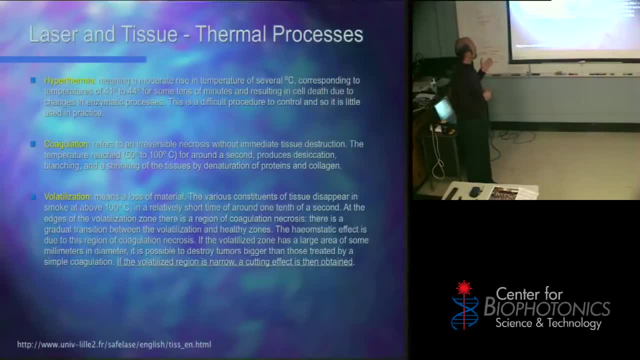 Excessive heat. Excessive heat. So if I keep living tissue cells at 41 to 44 degrees centigrade for 10 minutes or more, I will get some cell death because I'm effectively shutting down some of the enzymatic processes that keep the cell alive. 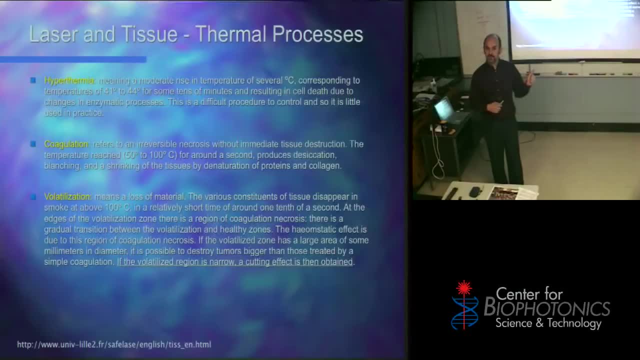 Okay, This is why we're worried about fevers. This is why we're worried that if your temperature is over 40 degrees centigrade for a long amount of time, you start getting delirious and it could actually kill you to get too hot. 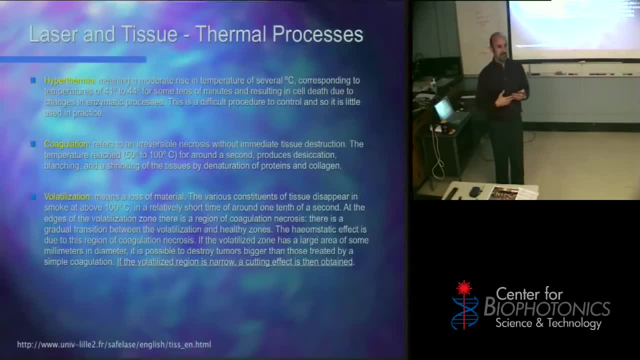 because you're basically shutting down your cell's processes in surviving. So that's kind of the one level of heating up things. Coagulation: It refers to irreversible necrosis without immediate tissue destruction. So necrosis is cell death. The temperatures reach 50 to 100 degrees centigrade. 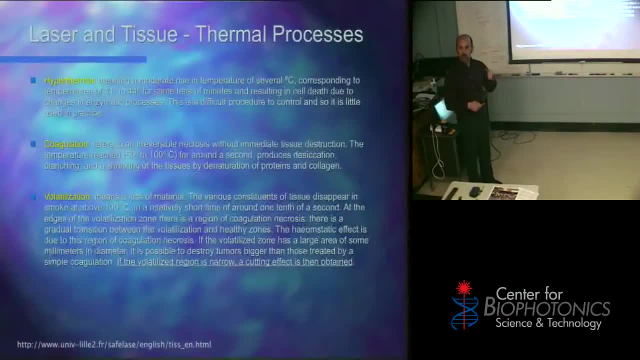 for around a second Produced desiccation. It means all the water is sucked out, Blanching and shrinking of the tissues by denaturing the proteins and collagen. So you guys ever cooked an egg? Okay, That gooey, clear stuff. 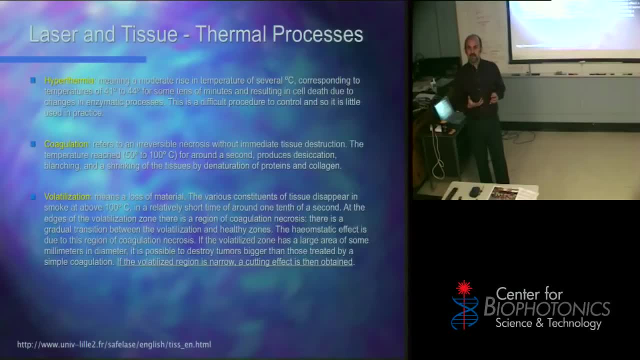 The moment it gets really hot, what does it do? Turns white. Okay, It coagulates. That's the same thing that happens to your tissues. Okay, The proteins inside them will turn like that And therefore they're no good anymore. 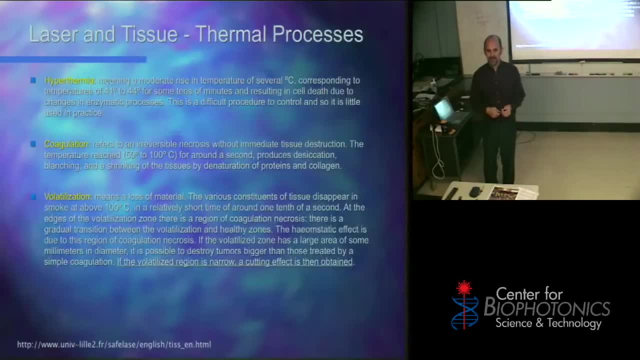 You can't use them. They might be edible, but they're no good to you anymore and to the living thing. Okay, And the last thing is volatilization. Volatilization means that you actually have material that's lost. 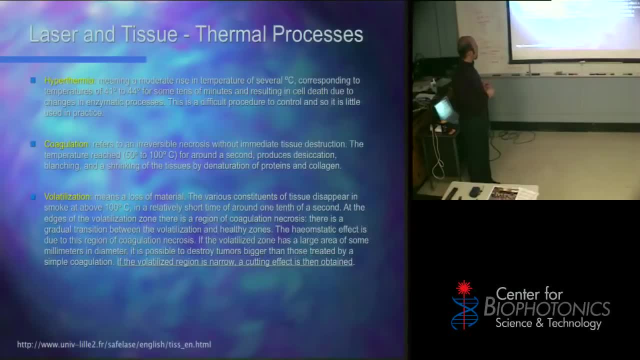 It vaporizes, It goes away. This usually happens above 100 degrees centigrade And it can happen very quickly, A tenth of a second or so. And again, if I were to shine a laser powerful enough to cause volatilization. 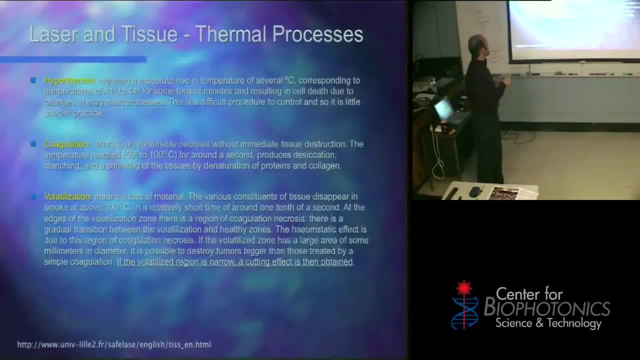 at the fringes, I'm also likely to get some coagulation And even further away, I'm likely to get hyperthermia. Okay, So these things compound on each other. See what I'm saying. If I get one little spot, really hot. 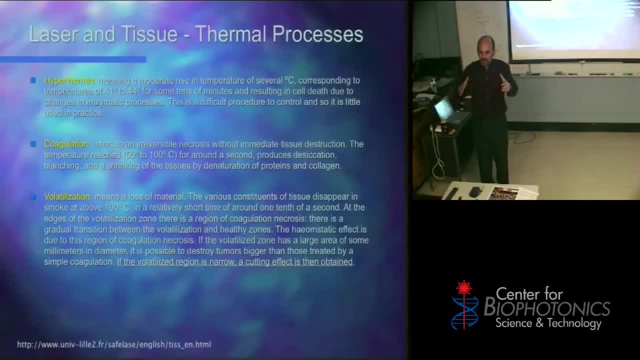 nearby it's going to get kind of hot, And even a little further out it's going to get warm. So you have to think Yes, Oh, yeah, Yeah, We're going to be talking about it, Lasix. 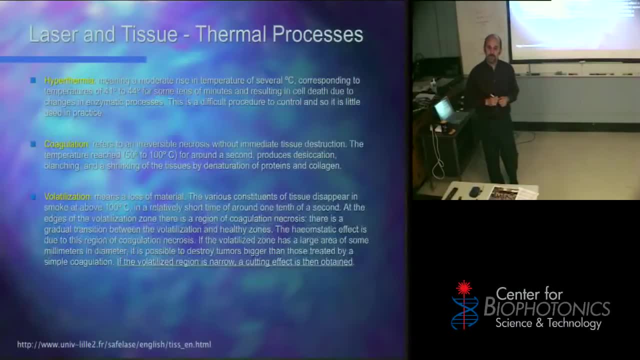 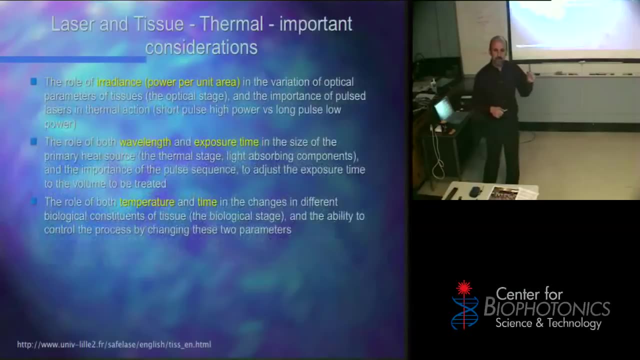 for example, And also whenever you use a laser as a scalpel. Yeah, Definitely Okay. So the thing we want to think about now, when lasers are interacting with tissue, is: we want to think about how much power per unit area is the laser delivering. 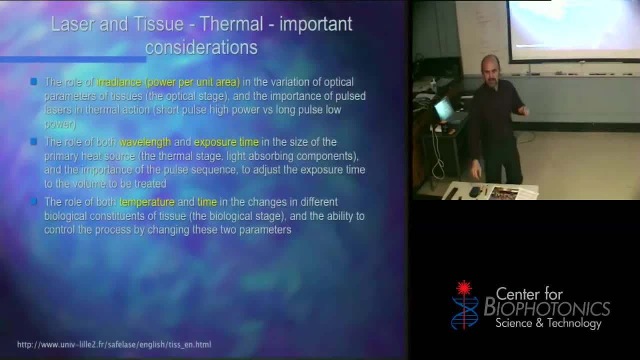 Okay, Because you can imagine a laser that has a certain power but it delivers it over a spot this big. How will that differ if that same power is delivered to a spot this big? What would cause, let's say that that laser has all that power? 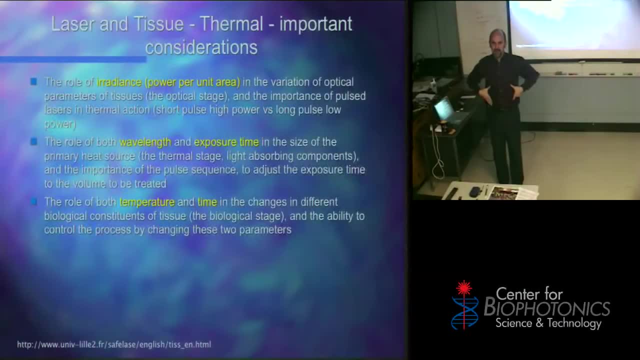 and it's delivering it to my stomach. Now somebody focuses all that power into a little one millimeter spot. What might the difference be in the effect on my stomach, on my tissue? Same power delivered over this much space, or delivered over this much space. 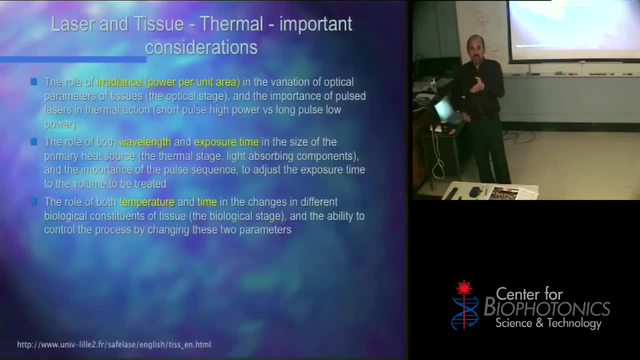 Well, it might keep you in there. potentially it would did you guys. I know this is kind of cruel. did you ever take a magnifying lens to the sun and try to fry a little ant? has anyone ever done that? ok, some people are willing to admit it. 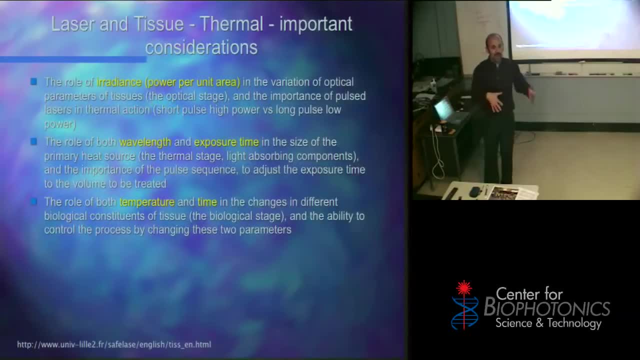 ok, now the sun by itself, the ants walking around. if I take that much of the sun, or whatever my size of my lens is and I concentrate it to a little point, that's the same power. but now it's concentrated on a little tiny point and the ant fries. 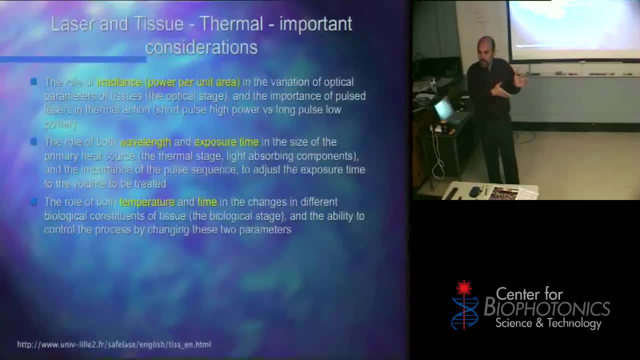 ok, or you can do it with paper. you burn paper. if my, if I take that magnifying lens and I don't focus it, I just keep it defocused. so the spot is large, all that energy is still there, but it's in a larger area the moment I focus it. 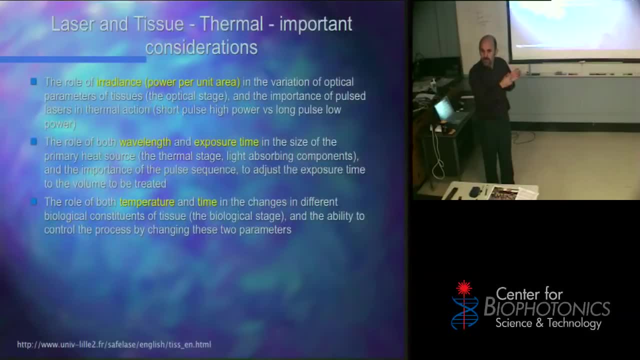 it gets focused down into one little spot and the paper starts to burn. ok, same thing with lasers. if I take a laser of a given power and I focus it down, it's a lot more powerful. it can cause a lot more damage. so the other thing that's important: 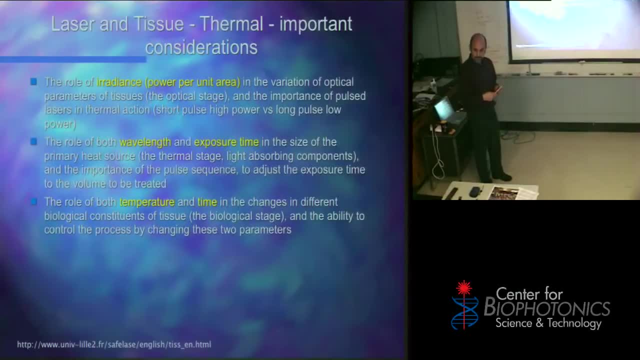 when we're thinking about laser interacting with tissue, is the wavelength. why might the wavelength matter? yes, it affects what tissue is actually absorbing it. yes, it affects what's going to be absorbing it exactly. very good, and how about? how could the exposure time affect things? 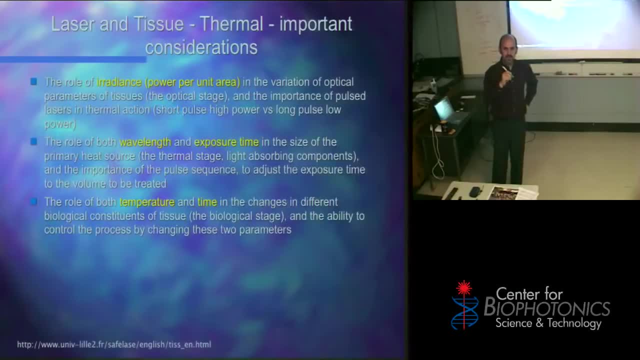 so if I got my laser on there for a second or if I got my laser on there for 10 minutes, how could that affect things? yes, the damage. or if the damage isn't cumulative, the effect is cumulative. so if you have more attack over a longer period of time. 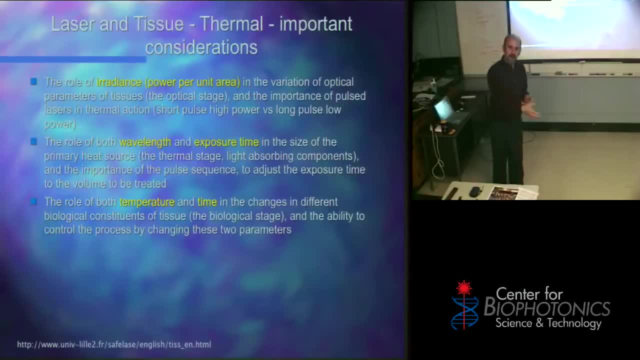 it's possible to affect. you're basically depositing more photons into that tissue. ok, if that tissue is able to absorb those photons, then you get a greater effect. now, if it's already pulsed away and there's nothing there, then it doesn't matter. but if it's still able, 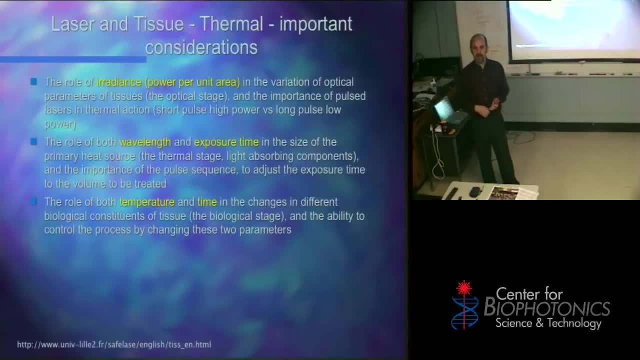 to absorb the photons, then you're actually increasing whatever effect you're getting on the tissue and these things- the wavelength and exposure time and power per unit area- affect the temperature right of the tissue and we know that the temperature of the tissue has a big difference. 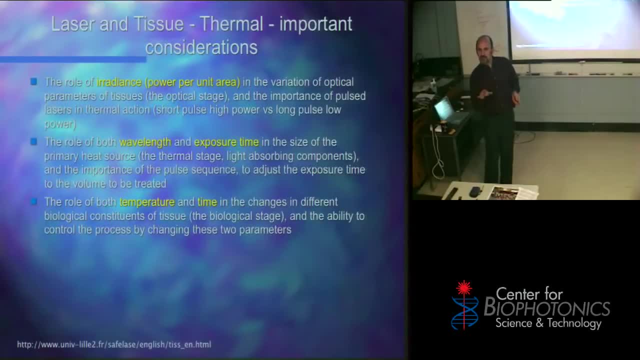 on what happens to the tissue. if it's kind of in the 40 centigrade, 41 to 44, things start to slowly shut down. if it's more like 50 to 100 centigrade, things start to coagulate. it's even above. 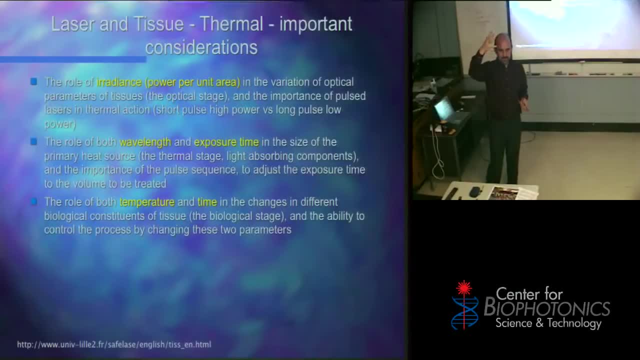 100 degrees centigrade you might have things vaporizing ok, and again that temperature over time. those two things affect each other, because I can heat something a little bit if I shine it for longer, longer, longer you can heat it more and more and more and it can lead to. 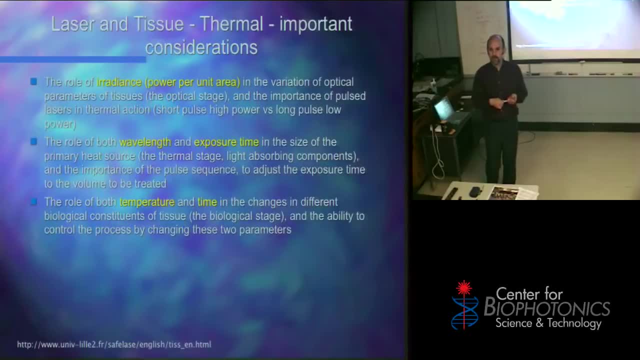 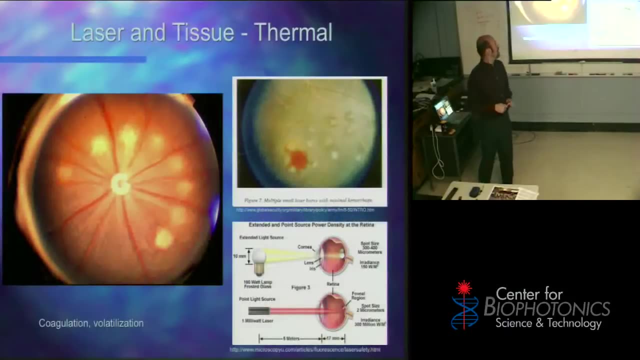 greater and greater damage. ok, now let's look at some examples of these types of damage. this is thermal damage. ok, primarily, things got heated up too much, too fast and caused some element, some cells, to die. this is a poor, unfortunate eye that stared at the laser a couple too many times. 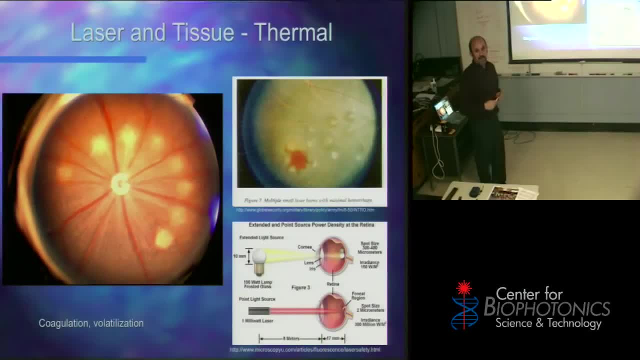 actually 1,, 2,, 3,, 4,, 5,, 6,, 7,, 8 times, ok, and the laser happened to be in different spots of the field of view, slightly different angles coming at it, and that's how you get. 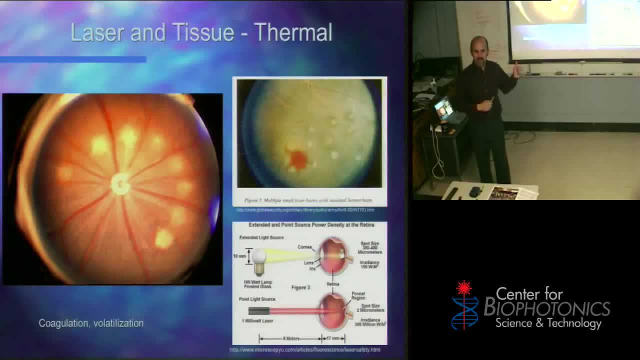 all these nice little patterns. this happens to graduate students every once in a while- hopefully never, but it does happen every once in a while that you get this kind of damage. here's small laser burns and a little hemorrhage that got caused by one of the couple of the laser burns. 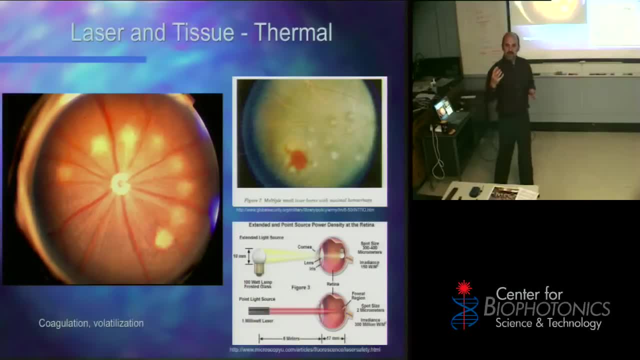 here you see more spots. ok, undergraduates and graduate students working with lasers have to always wear their eye wear, their safety eye wear because what happens is you tend to work with lasers that are not visible, tend to work with infrared lasers a lot, or you might work. 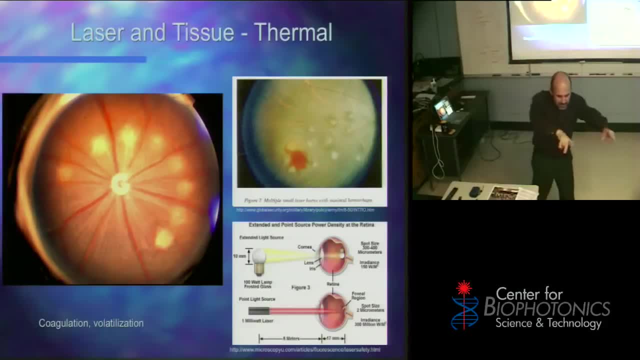 with an ultraviolet laser. ok, and what that means is you've got all these little mirrors lined up on your table and these little magnifying lenses and all these different things- reflectors, wave retarders, there's all kinds of things. I mean there literally could be hundreds of things. 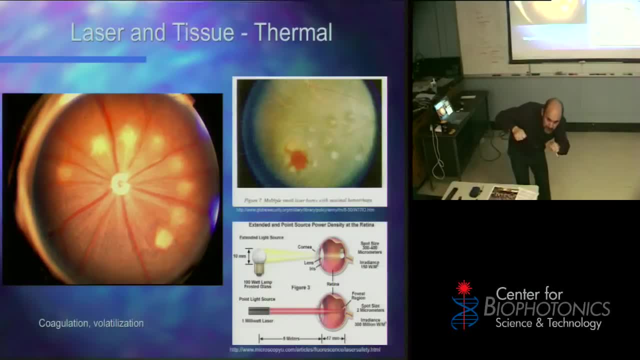 on one of these optics tables and you're aligning them and you see them and you're like, oops, I just moved the mirror and it shined in my eye and I just burnt a hole in my retina. ok, not so nice now that kind of damage. 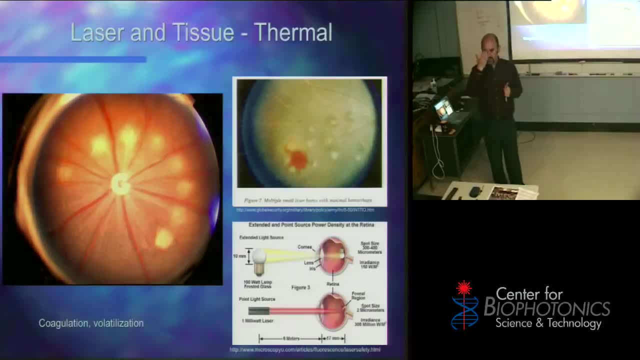 happens a lot with infrared. it doesn't happen so much with ultraviolet because the surface of your eye will block the ultraviolet. but this can happen and the difference is this. so, if you think about it, if you take a 100 watt lamp, you know your little incandescent lamp. 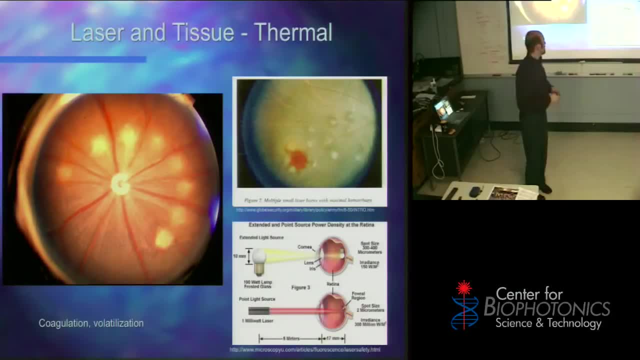 100 watts, pretty bright, right, kind of annoying bugs your eye. but the size of the lamp, let's say you've even got a pretty small one. you've got a pretty concentrated bulb. ok, that's only 10 millimeters. that means you've got a pretty concentrated bulb. 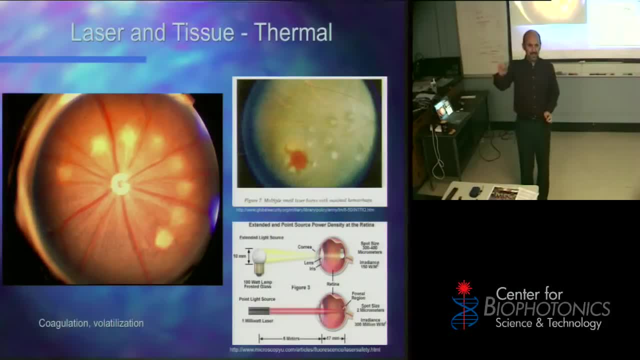 like this. that's 100 watts. that's like one of those halogen lights- really bright, you know, remember little tiny bulbs really bright. your eye has a lens to focus the light. it focuses the light and the spot size that happens on your retina is around 300 to 400 micrometers. 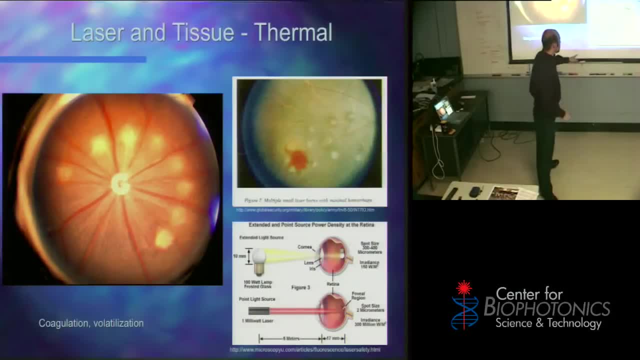 the focus, focus point on your eye. ok, if the light is about 5 meters away, so you're getting. you know, something less than a millimeter in size spot on your retina of that light bulb and that's registering as, oh, that's a bright light. it's kind of bugging my eye. 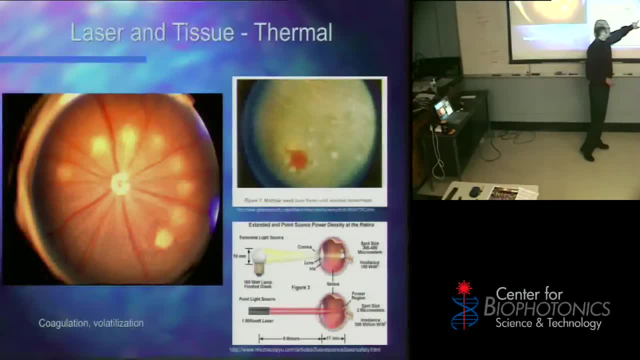 and that is about 150 watts per square meter. that's the amount of power delivered into your eye, 150 watts per square meter. now, if I take a 1 milliwatt laser, and this happens to be a 5 milliwatt laser- ok, so 5 times as much energy. 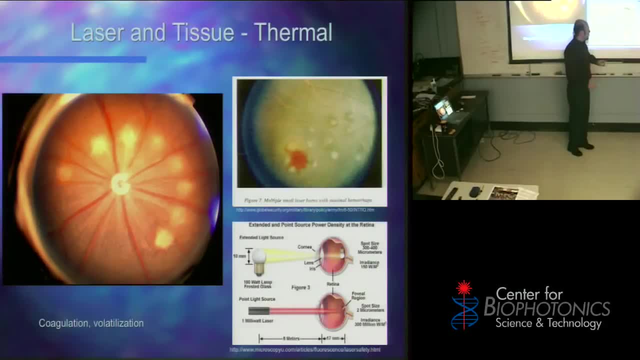 and I shove it into the eye from 5 meters, I get a spot that's focused on the eye of 2 micrometers. notice this will speak to 400, 2 micrometers. so now I've concentrated 1 milliwatt. this was 100 watts. 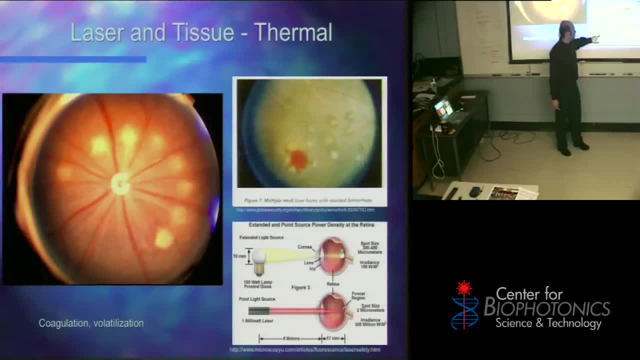 ok, this is 1 milliwatt, much, much smaller. I've concentrated it into a very, very, very small spot. the irradiance is now 300 million watts per square meter. ok, so, even though my original source was not nearly as powerful, it was all the laser has the one thing. 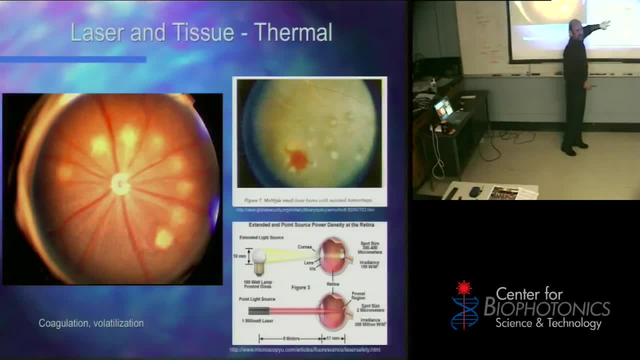 that delivers all that power directly, ok, like this radiates it out all over the place? ok. and the way the eye focuses and makes the spots eye, you can get damage. that's why we tell you not to stare at these. you won't get it very quickly. 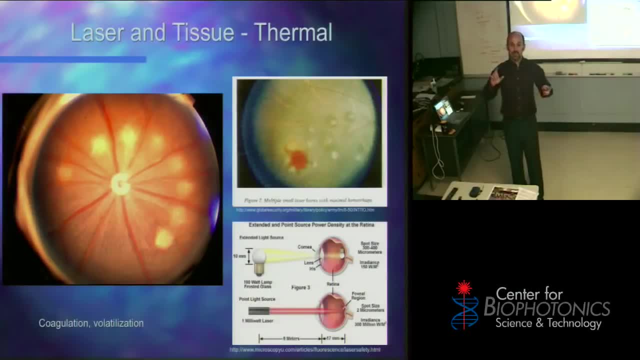 but it's just not a good idea. ok, and again it has to do with. so this is the main message: that the 2 sources can be. even the weaker source, if it's focused to a really, really small spot, can have a much greater potential for damage. 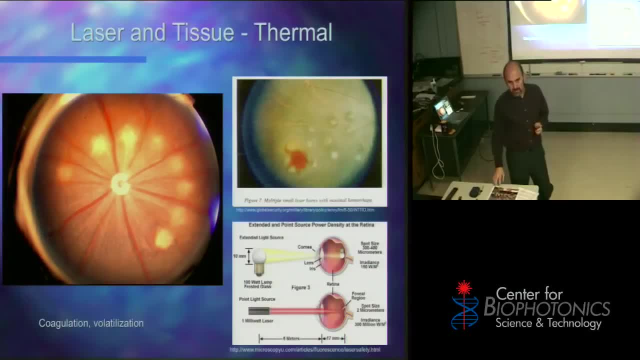 yes, there's a question I was just wondering with this specific picture right here where the person got like 8 pieces of damage, like to what extent is that damage? is this person now blind or do they just not see quite as well? because that seems like really horrific. 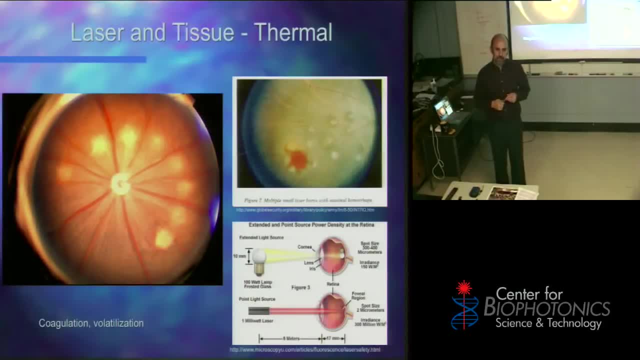 like: oh my goodness, 8 pieces of damage in my eye. did you go ahead? how bad is it? basically, ok you ever. you know, you guys know you have a blind spot in your vision. it's about the size of a quarter at about arm's length. it's a spot. 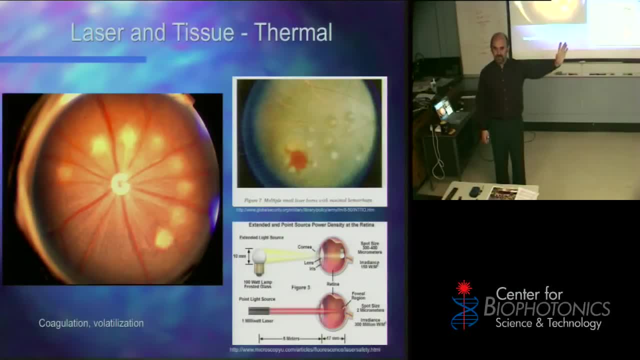 that your brain makes up, ok, just totally makes it up. ok, this person now has to make up 8 of those, this person's brain, ok, so, and that's bigger than the size of a quarter. so it's probably about- probably about- spots like this at this distance. 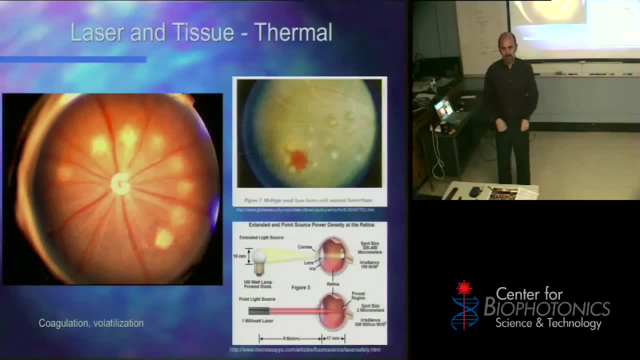 and they have 8 of them that they have to make up. so probably hampered, quite a bit hampered, and what they heard when this happened is they heard snap crackle pop, because basically it was like when you take the egg white and you take the egg white. 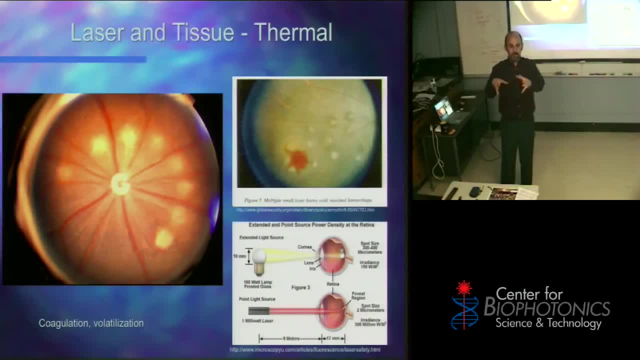 and you stick it on a really hot pan, you hear that whoop. you know it kind of makes that little noise as it congeals. that's what they heard here. these cells basically popped, they overheated and popped. yeah, so all the amylose damage spots came from. 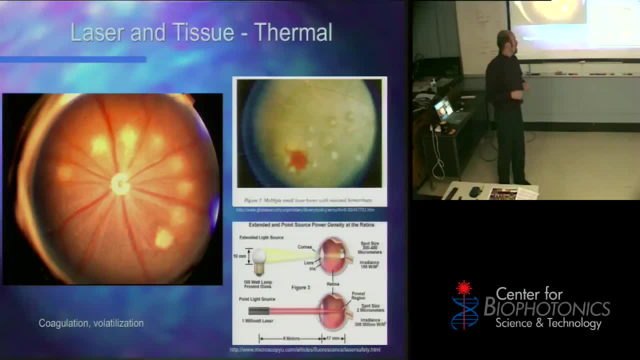 single point iron, or was it like 8 instances or not? you know, what tends to happen is there are experiments where you create arrays of lasers, so probably what happened here is there was something that was radiating out in a couple of different directions at the same time. 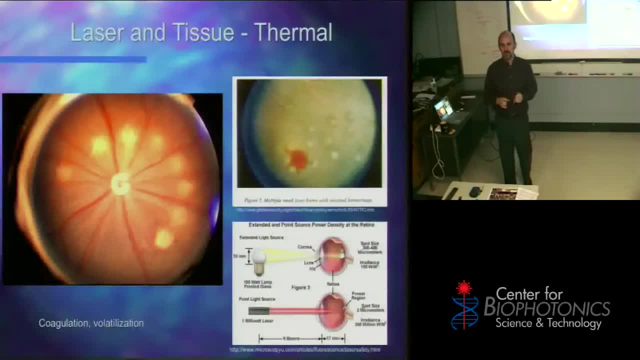 so probably it is one incident where it all came about, correct? yeah, because when I do this sometimes it's annoying. I mean, looking at it, it's kind of bright, but it's already spread out quite a bit. okay, it's already spread out more than if I just 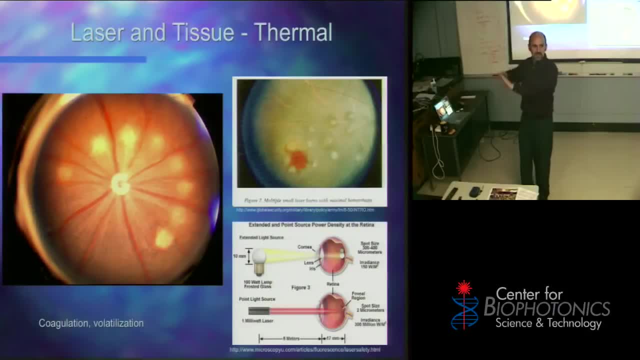 were to do this, and it's also being diffracted. it's scattering all over the place, so I'm not getting all the energy coming back to my eye. it's really going all over the place. yes, the good news is that most of us are smart enough. 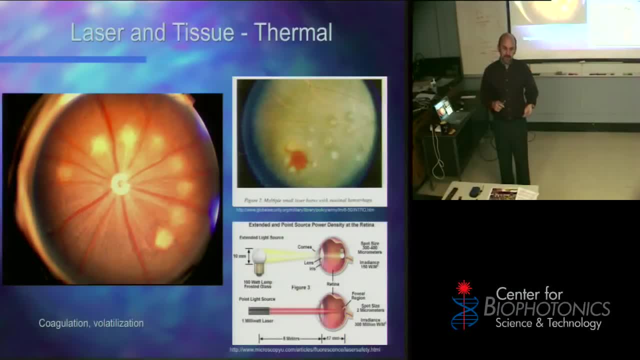 that when we see a laser like that coming to our eye, we close our lid and the response time that we have is fast enough that we don't cause damage it. it very, very mildly and again scatters and is mostly blocked because remember what happened with my finger. 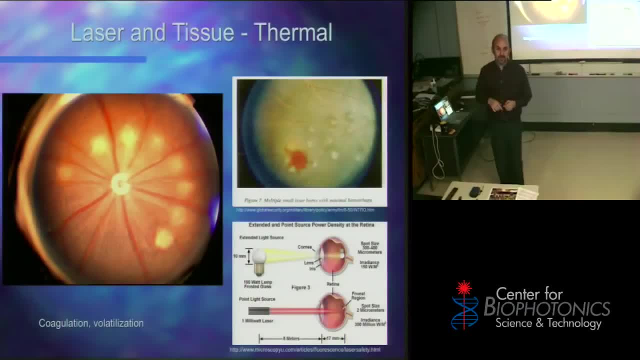 green doesn't go through very much. now the lid is thinner, so a little bit goes through, but much less. that's the other thing. it's a question of how much time you have to block out that. we're usually pretty good if we just turn away. just turn away. 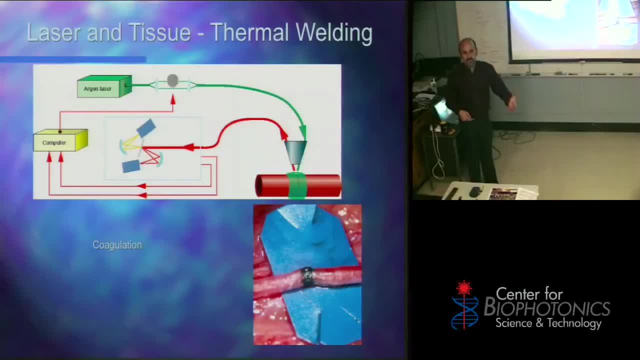 or close our eyes. that's usually what we do. the problem is when you can't see the laser beam, so another thing you can do is you can weld two tissues together. this is- I think this is pieces of aorta, and you can do this: weld it together. 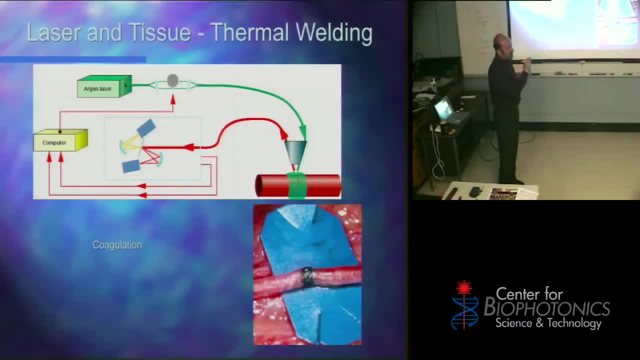 it's two vessels, just with coagulation, you can use the laser to heat up the junction and basically connect two vessels together. yes, well, what they did in this case is they actually put like a sugar on there and they caused that to coagulate. and then the idea is: 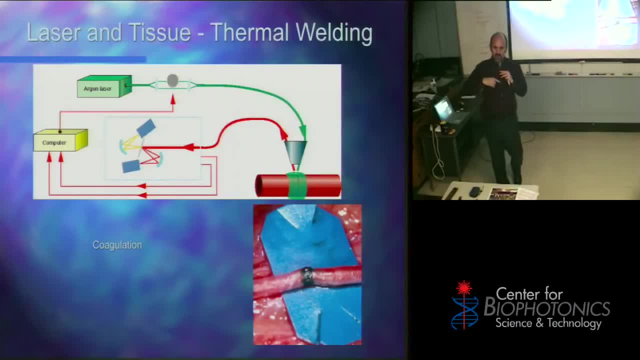 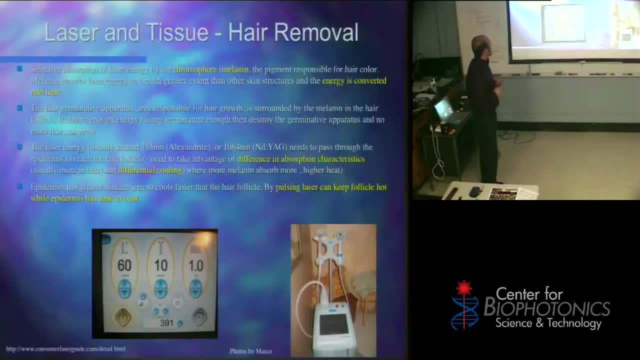 that the tissues, the two things will actually grow back together. so it kind of just forms a seal and then they can grow back. and this was the laser hair removal. and the laser hair removal they usually use around 755 nanometers or 1064 nanometers. 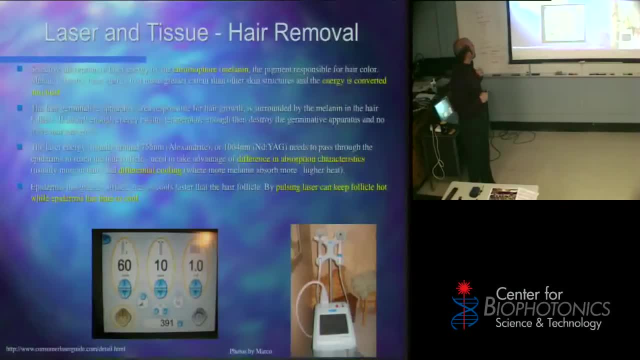 so those are both near infrared and what they're counting on is that that energy will be absorbed by your hair follicle. so those of you that have light colored hair- it's harder for light hair to absorb that energy. those of you that have dark colored hair- 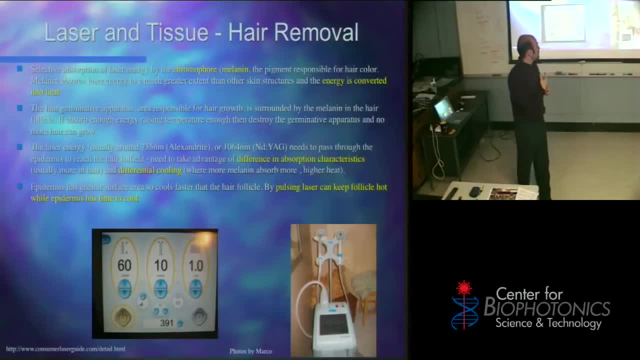 it's much easier for that hair to absorb the energy. so laser hair removal type of techniques work much better with people with dark hair. the lighter you go, the harder it is for that to work, just because I can't get very much energy absorbed by the hair follicle. 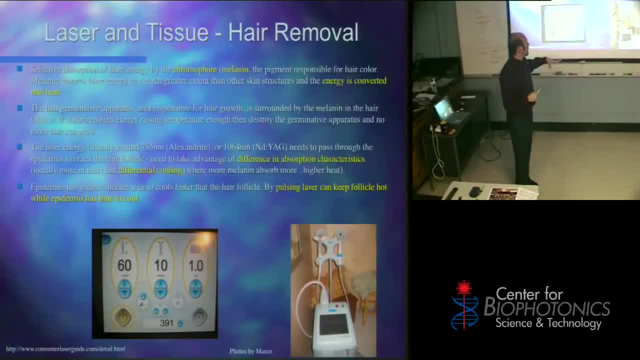 now the amount of time at which I do it. I pulse the laser so I can keep the follicle hot while the epidermis has time to cool, so this energy is also being absorbed by the skin. okay, layers of the skin, but if I pulse it, 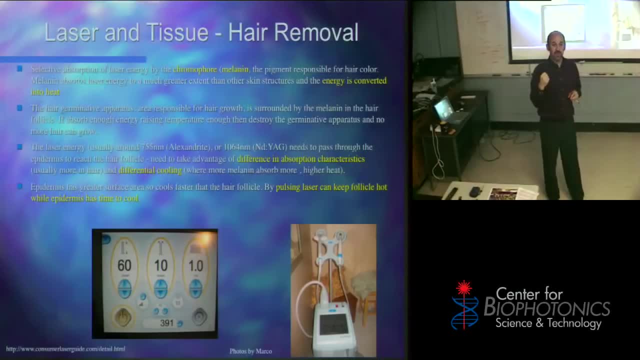 the energy, in a sense, has the most damage where it's absorbed the fastest and the most, which is in the hair follicle. so that's, and effectively I heat up that hair follicle enough that the cell that has the hair follicles, the cells around it. 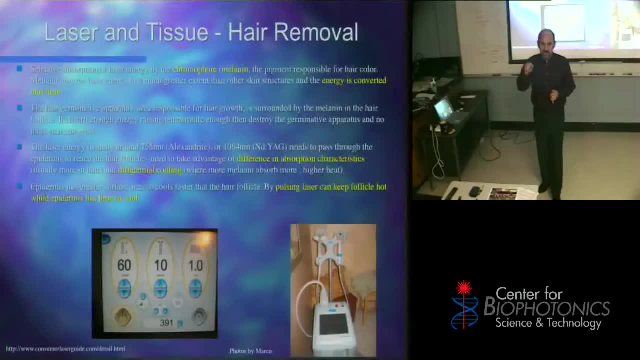 die. okay, that's what laser hair removal is: killing the hair follicle and the cells around the hair follicle. okay, does that make sense? the bad news is that in many states, you don't have to be certified to operate one of these, and there's this thing. 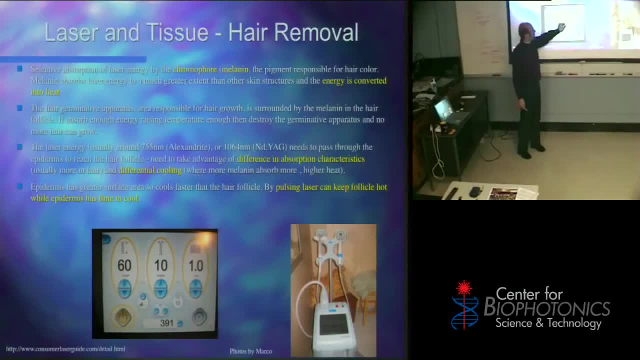 that tells me how long am I going to pulse the laser, at what power and how many times per second. okay, if they have those set wrong, they'll scar you, they'll burn you. okay, so ideally you want to know if somebody's been certified in using one of those machines. 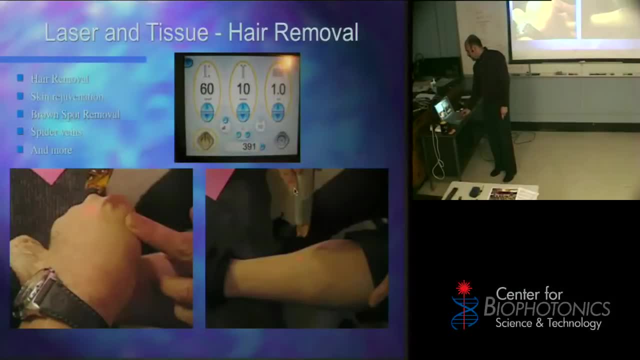 before you actually go and get that process done and you can do hair removal, skin rejuvenation, brown spot removal, spider veins. I can't remember. did I show you this video of me sacrificing a hair on my hand? I'll show it to you real quick, okay, so 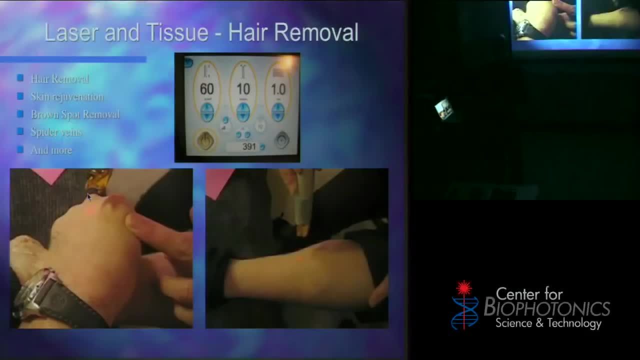 if you take a digital camera. now what wavelength did I say they use for hair removal? okay, 750 or 1000, those are near infrared, can our eyes see them, but my handy dandy digital camera can can't. so here I sacrifice the hair on my hand. 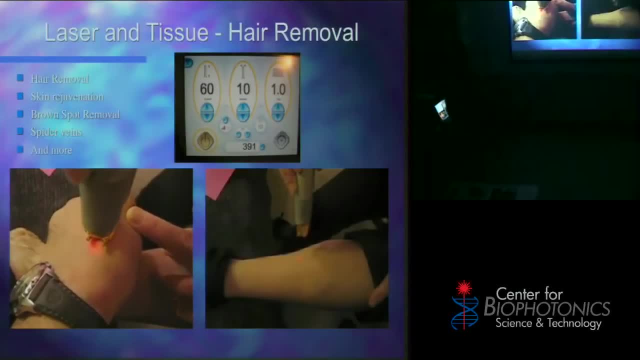 so first, what they do is they cool the hair, they put a little piece of metal that's cold and now watch. okay, that was it. you saw the flash. now, when I was in the room, I saw nothing. I saw nothing. I saw nothing, but that flash was the reflection. 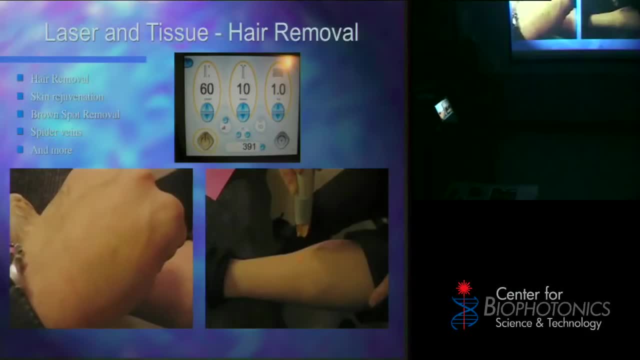 of the near infrared laser shining off of my hand, and that's the hair right there. I hadn't shaved it, so what it did is it singed the whole hair and it came back. I didn't want to really sacrifice it. I would have had to shave it. 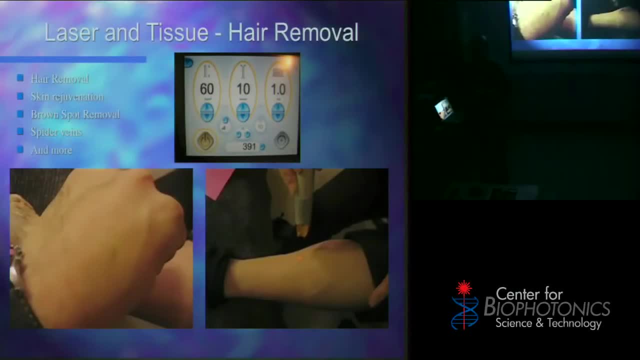 so that all the energy got concentrated in the follicle. but I didn't shave it, so all the energy got concentrated in the hair itself, destroyed the hair but didn't destroy the follicle. that's why they have you shave first before they do these laser hair removal procedures. 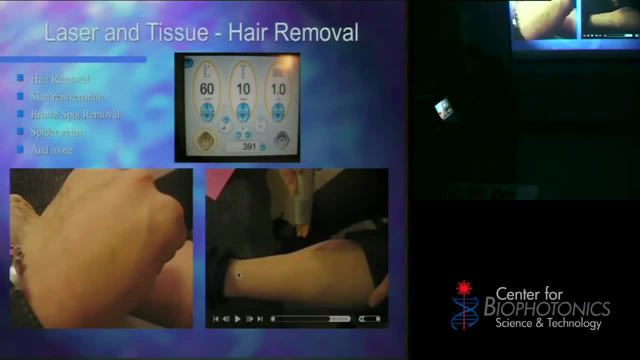 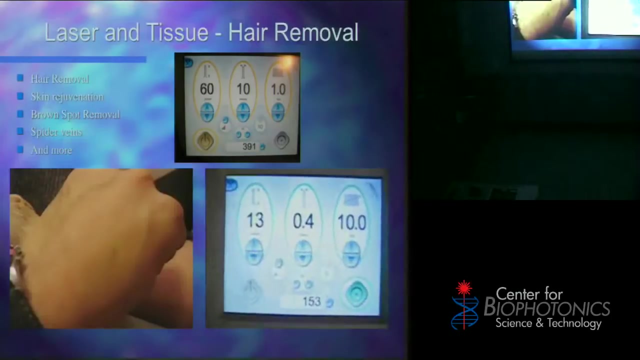 okay, and this is on a leg. this is for removing wrinkles, and you see all the flashes. that's the laser flashing again in the room. you can't see it, okay, but because I have the camera that can see the near infrared, I can see it reflecting. yes, 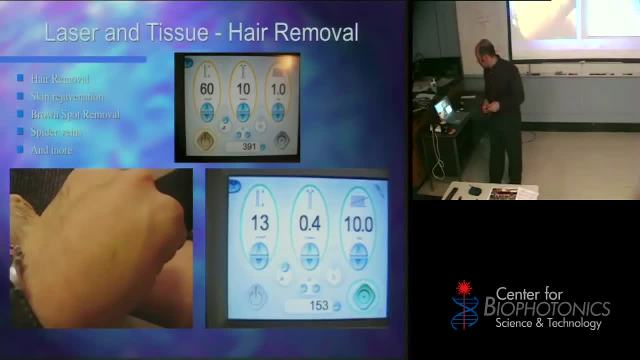 okay, the idea for removing the wrinkles is that basically I heat up the tissue and the collagen fibers kind of start to stretch and realign when they cool. they should stay that way. I mean, over time they'll come back. but yes, they do. they use it to remove. 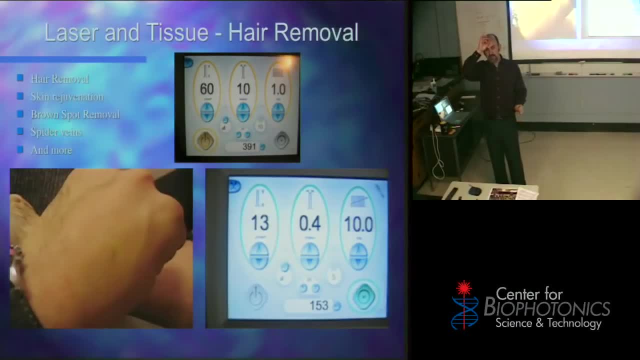 scar tissue. port wine stains like big red stains. I don't know if you guys, guys who even know who Gorbachev was- okay, Gorbachev used to have this big port red wine stain, those kinds of things. they remove it for that certain types of acne. 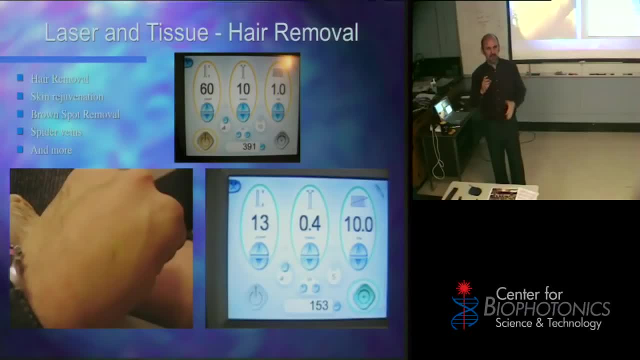 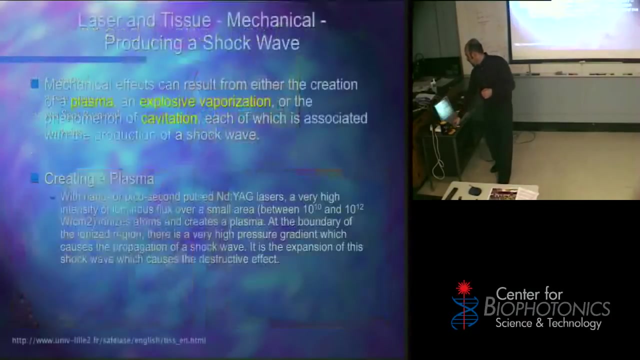 it can be used for. you know, it works best for things that are sealing of surface vessels, things like that. that's where it works best, and then that gets they kind of get closed, or for tightening. okay, now I'll go through a couple more of these you can also produce. 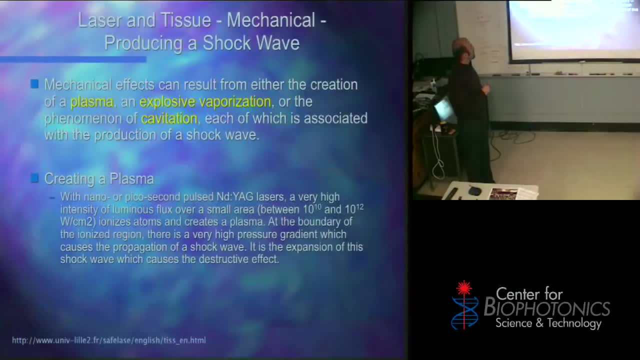 a plasma. you can bump enough energy with your laser that you cause basically an explosive, vaporization or cavitation. so you basically create a plasma with a laser and you can. you do it very, very quickly. you put a lot of energy in a very small spot, okay. 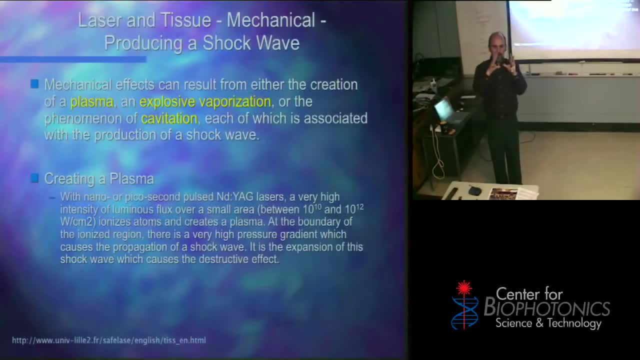 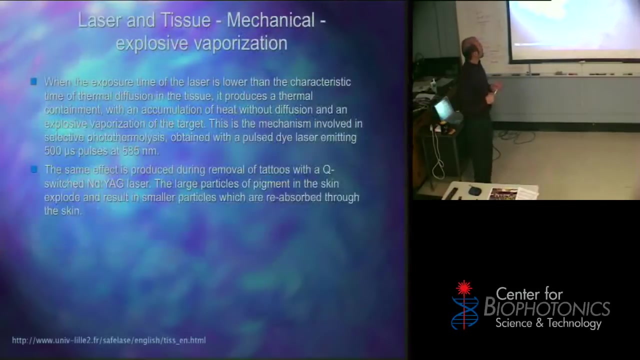 and what that does is it creates a quick bubble, but then, when it collapses, it creates a shockwave and it breaks things near it. okay, let me show you some more things here. with that I thought I had. okay, that explosive vaporization basically has to do with the fact that 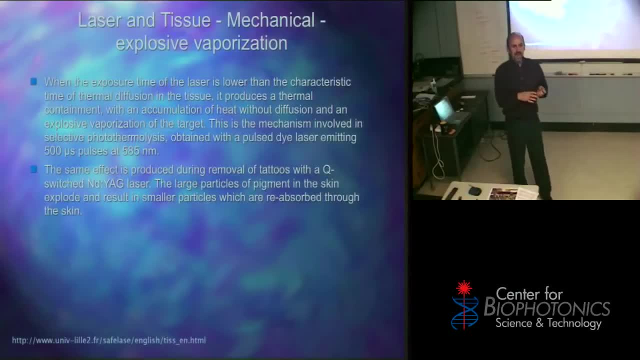 you have to get the energy into the system and it has to dissipate. when you turn it on, when you turn the laser off, that energy has to dissipate somewhere. and what it does is it basically causes the particle that it's near to break. and what do we use that for? 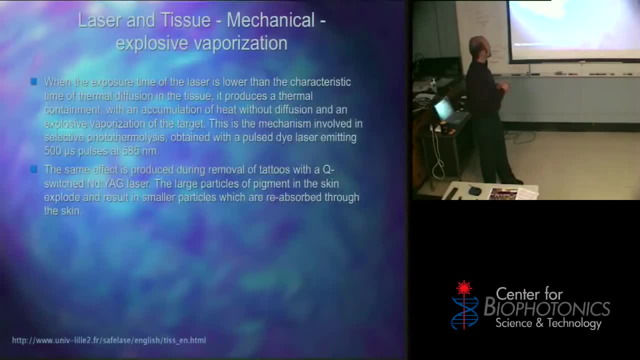 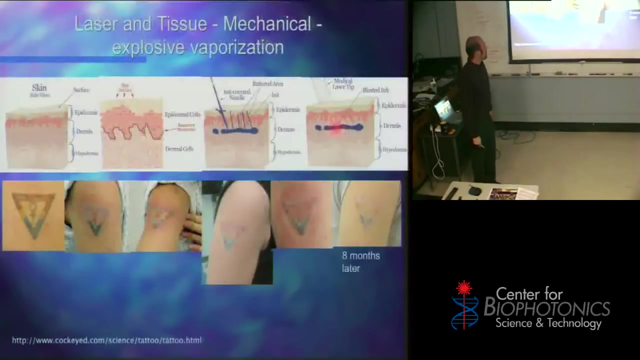 we use that to remove tattoos because the large particles of pigment in the skin explode, resulting in smaller particles, and your body absorbs those smaller particles and the tattoo is gone. okay, here's the example. this person went through a process of eight months to go out from that. 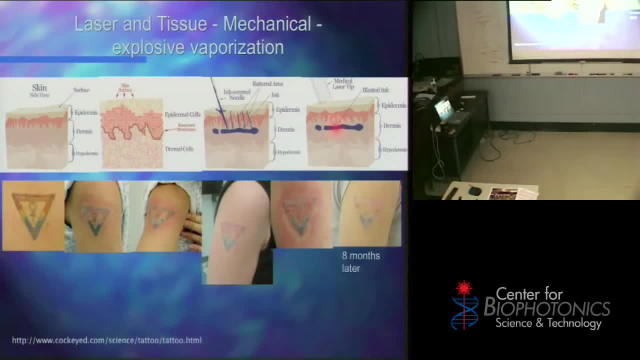 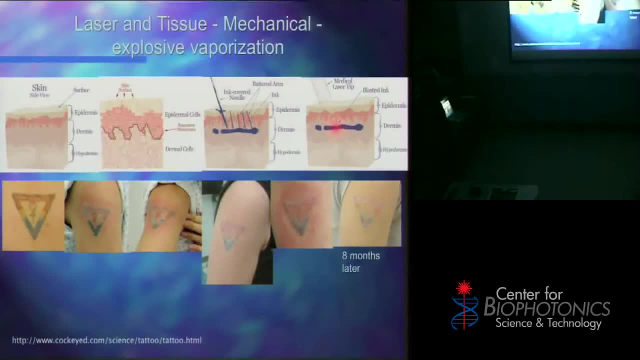 to this. okay, notice it isn't completely removed, it's, you know, somewhat removed. and notice that certain colors went away better than others. okay, like the red went away pretty well, the blue not quite as well, and the black in the center went away well, but what happens is: 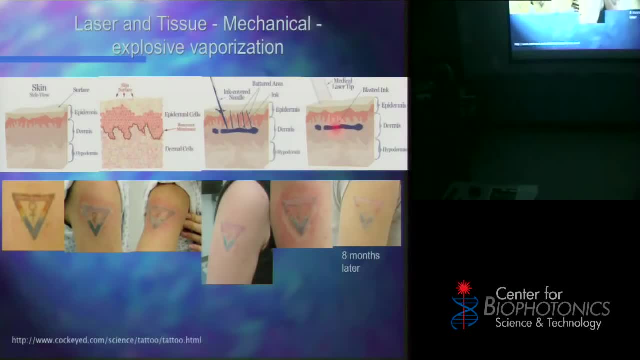 this is your skin. you have the surface, which is the epidermis, the dermis and the hypodermis, and what they basically do: we slough the skin, the surface, all the time. it comes and goes. that's why you put a temporary tattoo. so over time it's gone. 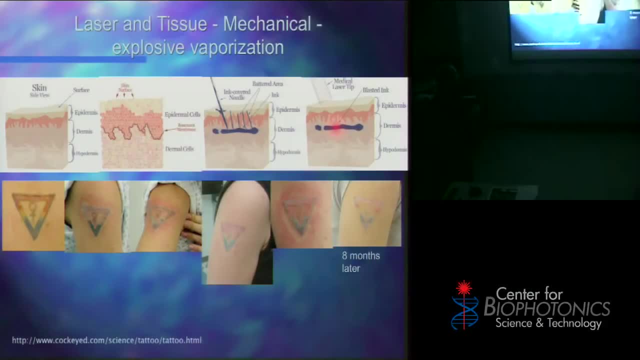 okay, or you wear it with a marker on your hand over time. it's gone. what they do when they make a tattoo is they take a little needle and they go underneath and deposit that into the dermis. the dermis doesn't get replaced. that's why it's permanent. 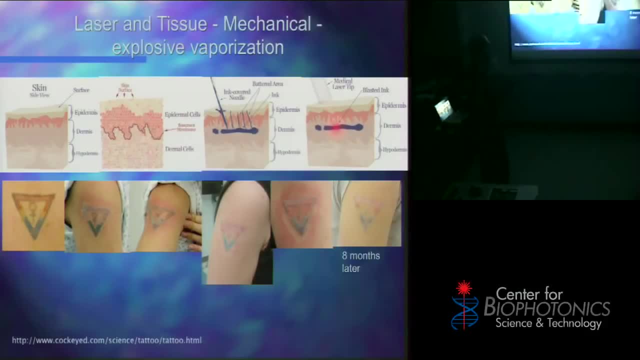 so when you want to get rid of it, you basically use a medical laser. it has to be absorbed by the epidermis and make it into the dermis and the energy has to be deposited in the epidermis, into the ink and the way you do it. 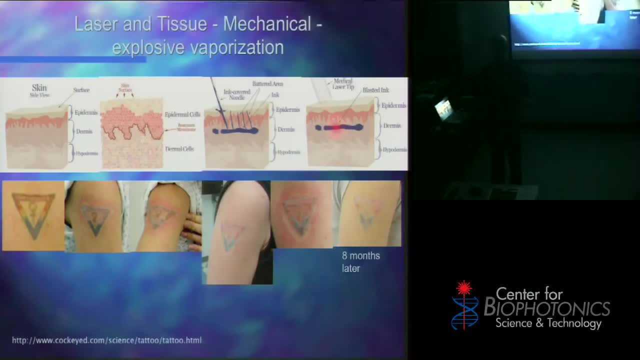 you do this explosive vaporization that causes the ink particles to blast into little pieces and then get reabsorbed by your body, but they do cause some scarring. I mean well, not so much scarring, but they do cause some temporary damage, as you're getting. 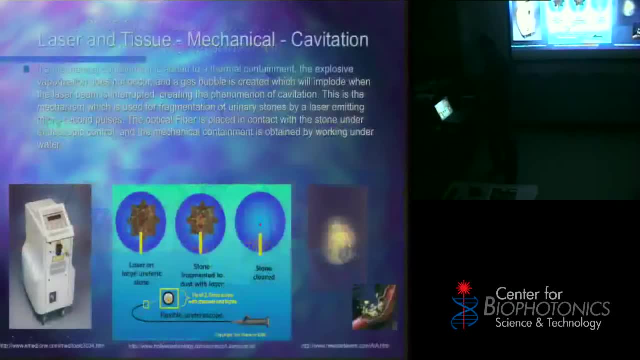 the process done. you can also use this cavitation to break stones, kidney stones. you can go inside with a fiber optic to where the stone is. you can go inside and make these fast pulses of the laser that again causes this cavitation, which causes the stone to break up into little pieces. 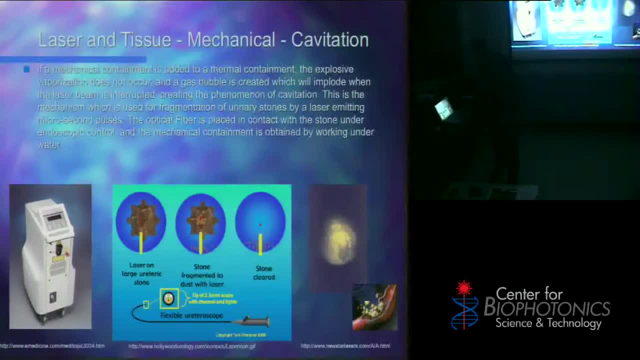 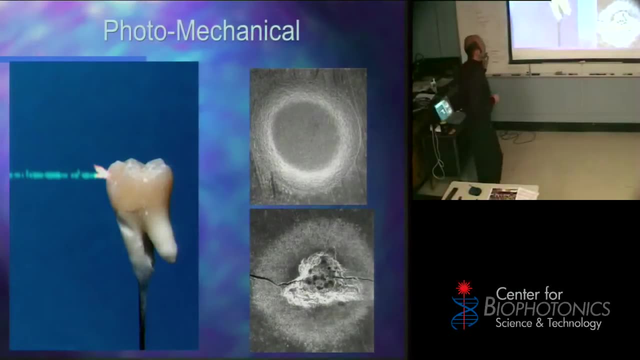 and hopefully the pieces are small enough they can flush through your system. now I can also use photomechanical, so in this case I can use a laser to remove stains on a tooth. but if I use too much power, this is what happens: I crack the enamel. 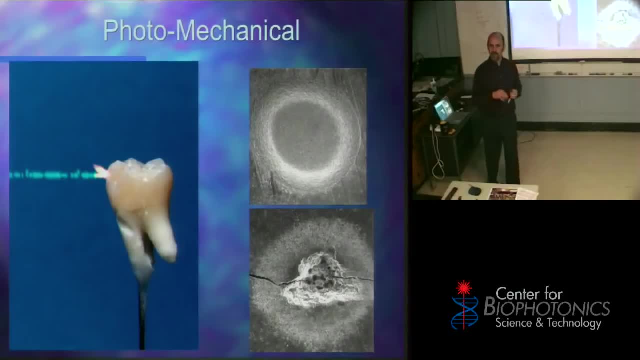 so this is where it's very important to deposit the right amount of power over the right amount of time, and it's going to depend on the surface. you can get this nice kind of mark like this or you can get this. that's all just depending on the amount of power delivered. 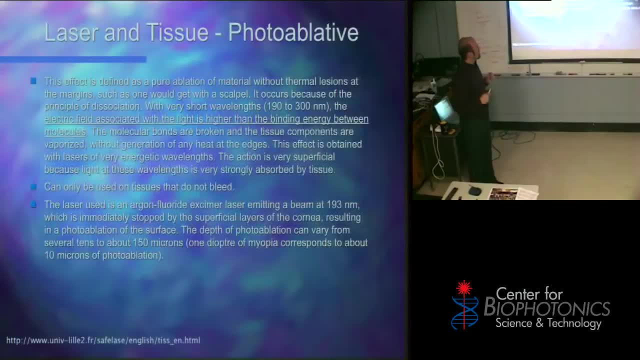 and then there's photoablative. photoablative takes advantage of the fact that if I put enough energy in there, I can make. if the electric field associated with the light is higher than the binding energy between molecules, I can make the molecules fall apart. this is that idea of ionizing radiation. 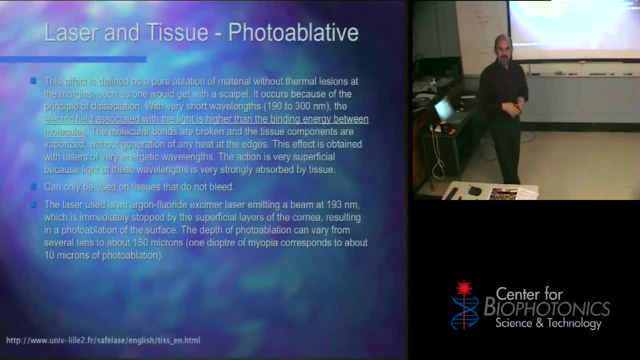 that we talked about on the very first day. if I have enough energy in there, I make the molecule and the atoms just basically fall apart. the electrons disappear, they go away, and so what happens is with that molecular bonds are broken and the components are vaporized without generation of any heat at the edges.